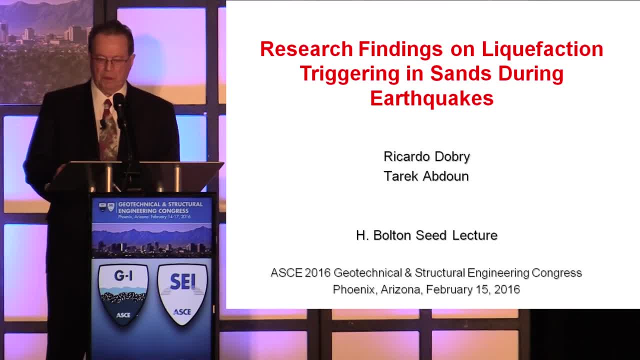 magnificent paper in 1971 on the simplified procedure. The method had stood so well the test of time that any new development on triggering tends to occur naturally within the framework of the simplified procedure. This is certainly the case with the findings I will be presenting. 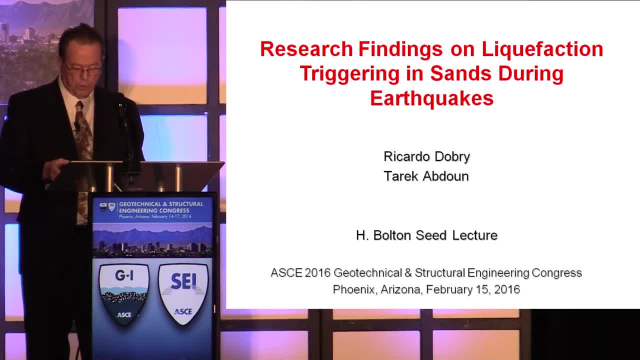 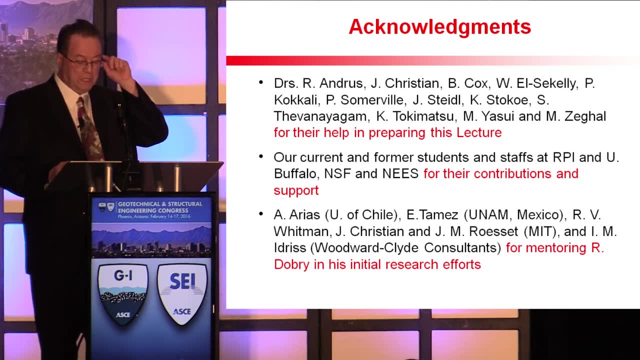 today, which are either extensions or proposed modifications of the simplified procedure. I also want to acknowledge the people and organizations listed on the screen for their support and help in preparing this lecture. Lots of people, I am not going to read all their names. I am not shy. Whenever I am in trouble, I reach. 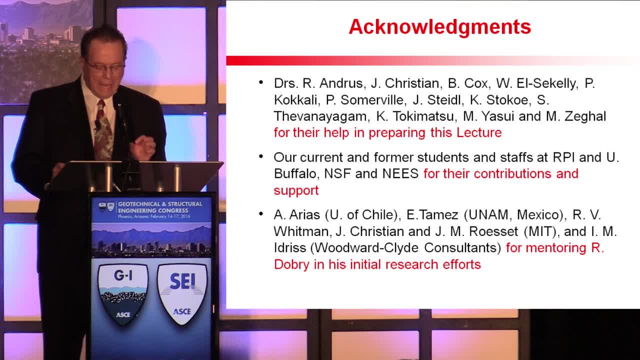 for the phone. Lots of people to say thank you, But let me add special thanks to six key people who played a major role in my professional career by mentoring my initial research efforts many years ago. They are Arturo Arias in Chile, Enrique Tamez in Mexico and 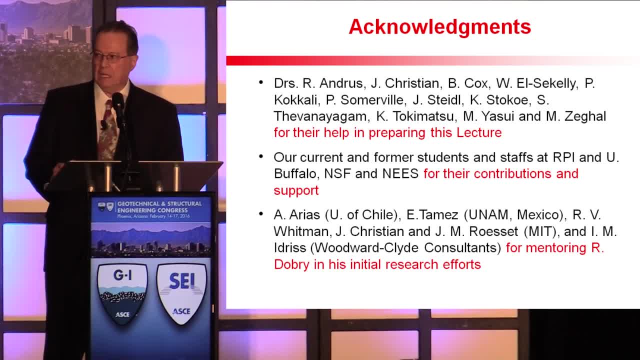 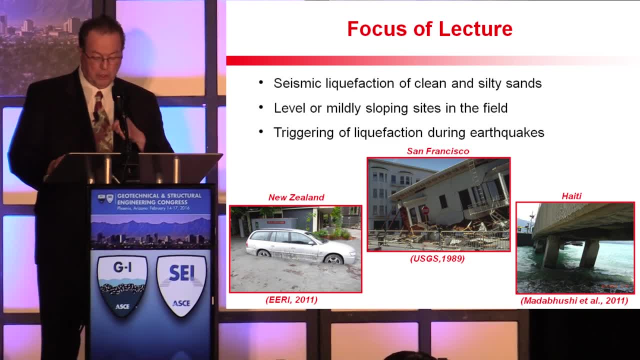 Bob Windman, John Christian José Roset and Eddie Idris in Colombia. Thank you. in the US, The three photos on the screen correspond to liquefaction effects on sands in New Zealand, San Francisco and Haiti. Liquefaction occurs in many large earthquakes with devastating effects, and it is also a 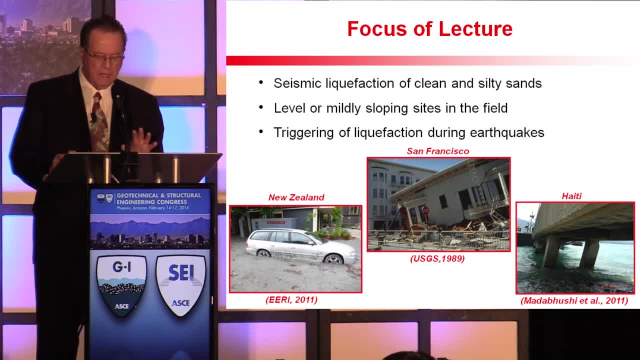 very complex phenomenon. These are the two main reasons why it keeps coming back at us and why we are still working on it after half a century of research. These three photos illustrate the consequences of liquefaction during earthquakes. My focus today is not necessarily on those consequences, but rather on the triggering. 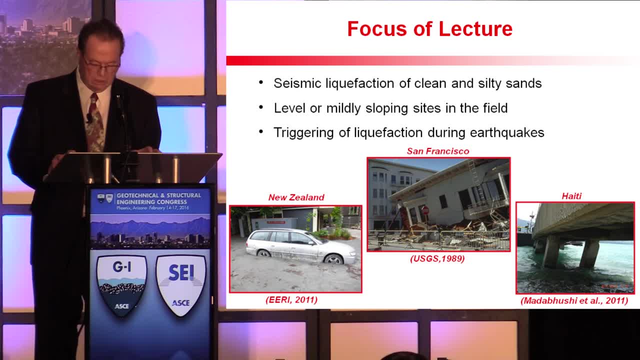 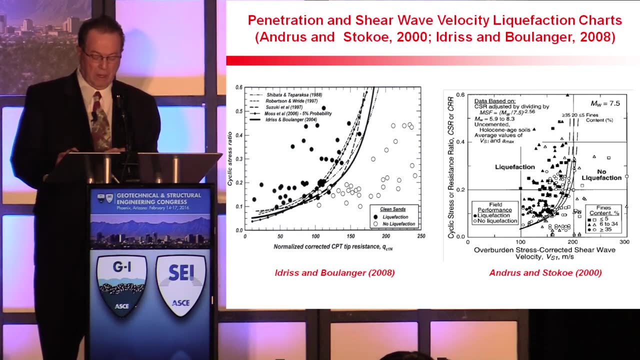 of liquefaction in level or almost level sites, with the consequences typically happening only after triggering has already happened. There have been a number of triggering events, Many liquefaction charts proposed over the years based on the simplified procedure, all calibrated by field case histories of liquefaction, and no liquefaction typically normalized. 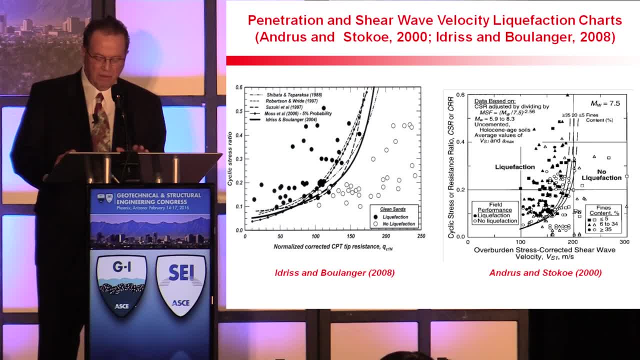 to earthquakes magnitude 7.5, and having the common format you see on the screen. Many of you are very familiar with these charts. The three main properties used to measure liquefaction resistance are: standard penetration resistance, or SPT, which I am not showing. static cone penetration resistance, or CPT. 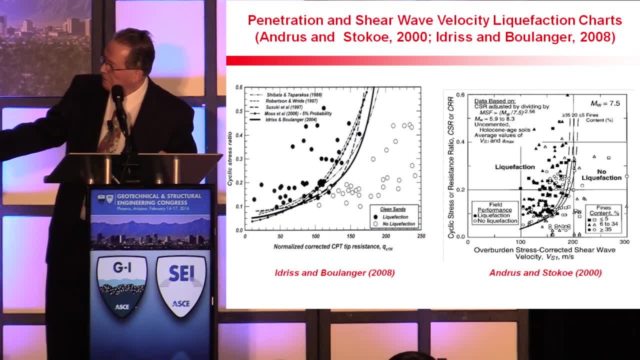 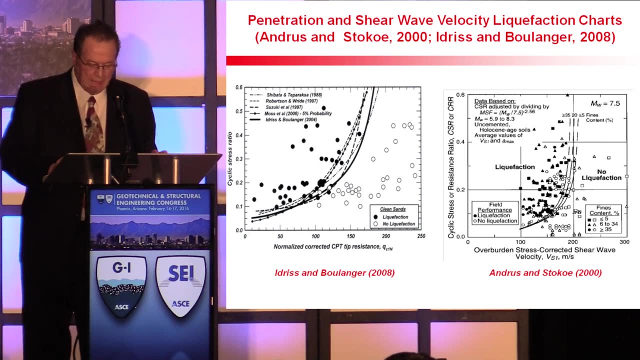 in this chart to your left, and shear wave velocity, or VS, in the other chart to your right. The parameter along the y-axis of all the charts that defines the seismic demand on the soil is the same in all of them: the cyclic stress ratio, or CSR. 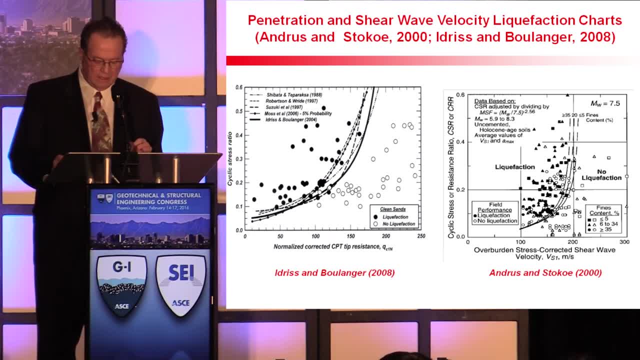 Let me add a couple of comments about the two charts on the screen. The CPT measures penetration resistance, so it is a large strain field test, while VS measures the soil shear stiffness at very small strains. Also, the case history is used to calibrate this particular CPT chart. 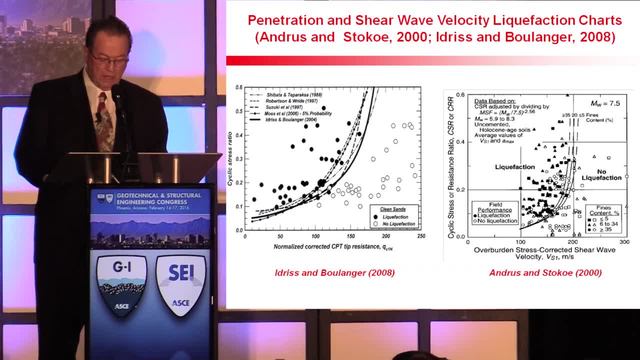 The CPT measures the pH of the soil, the pH of the soil and the pH of the soil in the soil at low levels, so that when it enters the soil it gets up to 7.3 grams, And the SPT measures the pH of the soil in the soil- 7.6 grams. 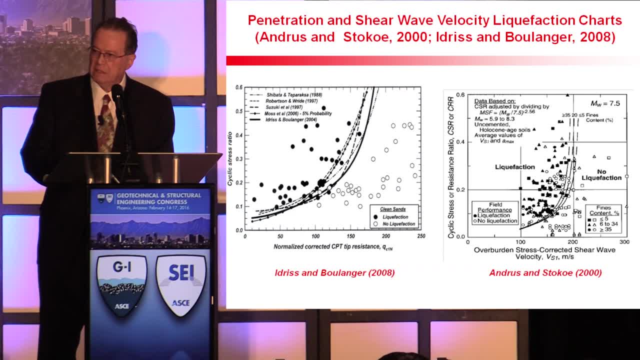 When the pH of the soil is higher, it loses its pH and then the pH is less and the pH of the soil is higher and the pH of the soil is less than their normal pH. On the left we see the clean sand. 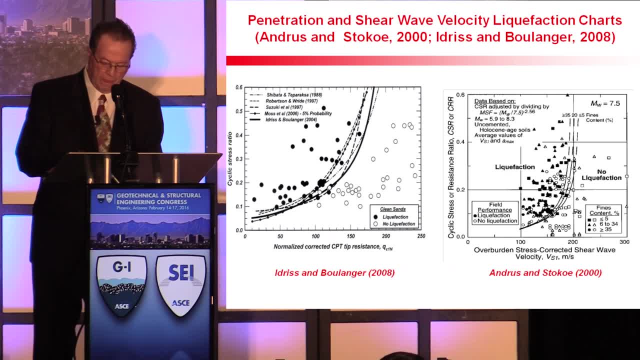 For the clean sand. the chart is only valid for clean sands having less than 5% or 6%. For silty sands, Idris and Boulanger and other authors have developed, for the CPT as well as the SPT, a fines correction which increases with the amount of fines and which is added. 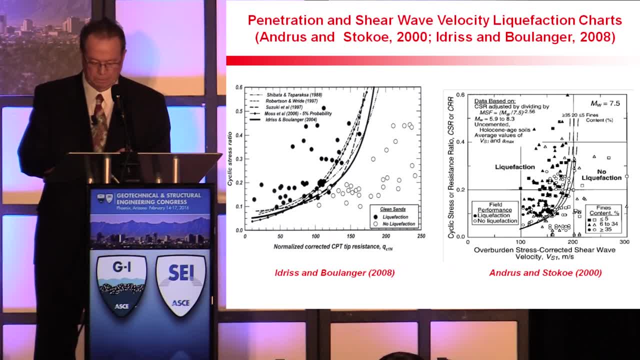 to the measure penetration resistance before entering the chart. resistance can be quite substantial. For the VS chart the situation is simpler, with the chart being essentially independent of the fines, so no correction is necessary. In the year 2000, Andrews and Suki tried to establish a difference by plotting these three curves, which I will point. 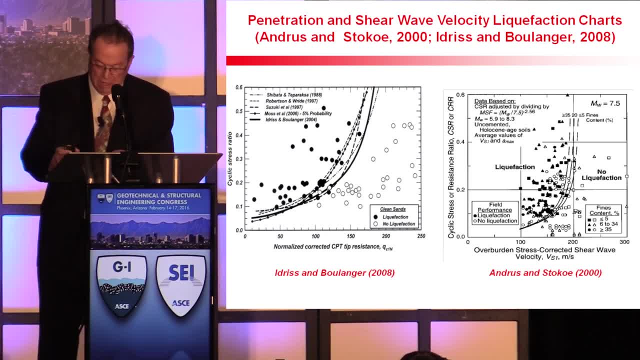 to you if I could, but I cannot, which depends on fines content. But as you can see, the three curves are very close and a more recent study by Kayen and his co-workers definitely proved that no fines correction is needed in silty sands- at least up to 35% fines when a shear wave velocity chart is used. 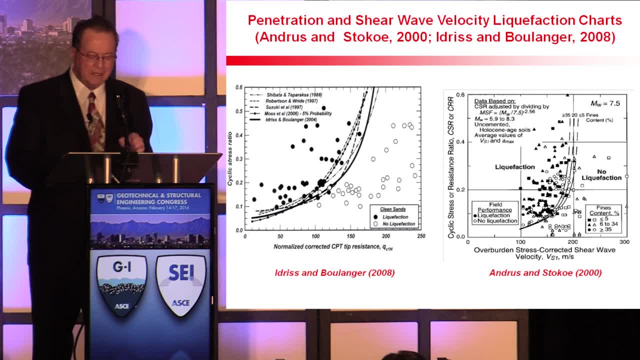 My final comment about these charts is the special role played by the cyclic stress ratio measure along the y-axis. This CSR is the cycle of the cycle of seismic demand, calculated for all the data points used to calibrate the charts corresponding to sites that have liquefied or have not liquefied. It is also the y-value you will use to plot your 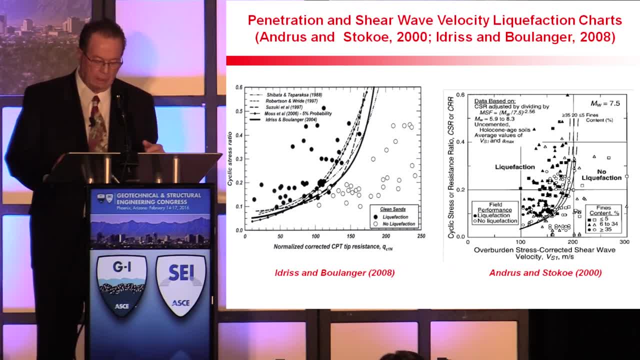 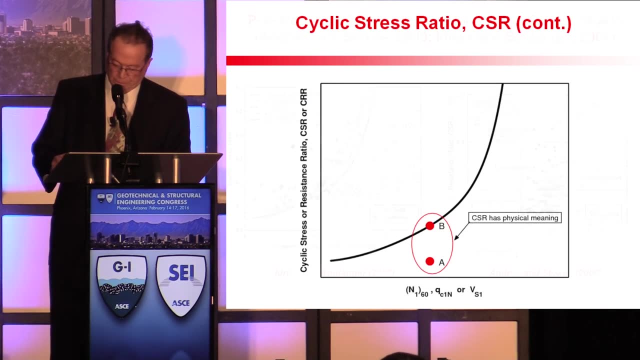 site when evaluating liquefaction potential for your design. earthquake CSR is a measure of the cyclic shear stresses imposed by the earthquake on the liquefiable layer, and it is usually calculated from the peak ground acceleration of the earthquake. Now, due to the difficulties involving trying to define the ground acceleration at a site which is liquefying in the simplified method, this acceleration, as well as the CSR, are defined not for the actual site and layer, but instead they correspond to a fictitious similar site equal in every respect to the original one, except that it does not build up or pressures in any layer, and thus the CSR is not designed to be used for the actual site and layer. 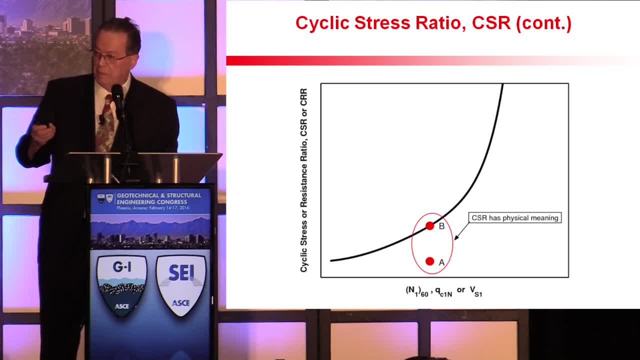 and is assumed not to liquefy. for the purpose of estimating CSR, This is equivalent to assume that the seismic shear stress and strains acting on the liquefiable layer are not affected by the strain softening which invariably occurs during pore pressure buildup and liquefaction. 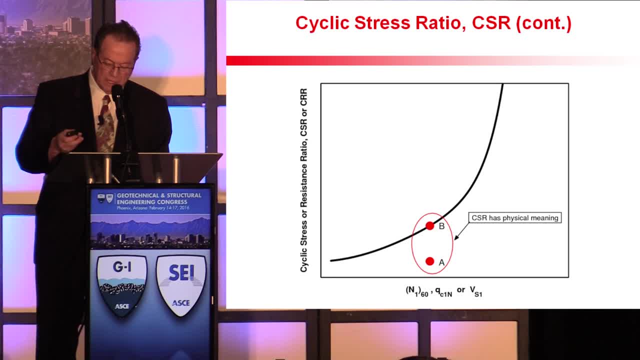 For the sake of simplicity, the method neglects this softening of the liquefiable soil layer induced by the pore pressure buildup And all your calculated accelerations. shear stresses and shear strains are index properties without physical meaning if the soil liquefies. 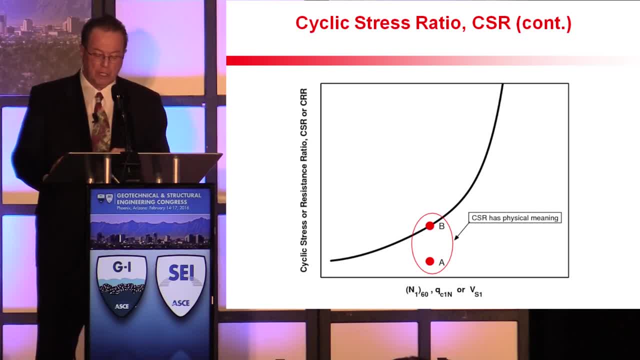 In other words, if the point of the chart corresponding to your site plots below or on the curve, that is, point A or point B in the figure. these calculated values of CSR shear stress acceleration are reasonable representations of the actual rate. 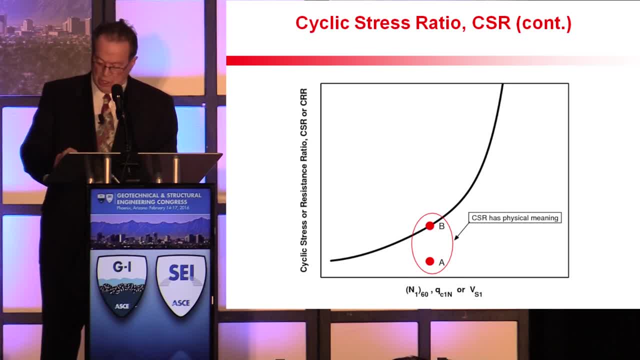 and the actual values developed in the soil during the shaking. On the other hand, at point C, the calculated CSR- shear stress acceleration strain- have little to do with the actual values and in this case CSR is an index parameter without physical meaning for the site. 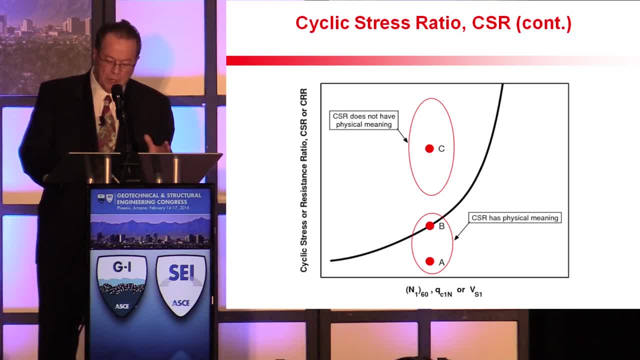 I'm not criticizing this at all, just clarifying the issue because I will need to come back to it later in the talk. In fact, this simplification seems to be unavoidable in the process of making the process truly simple and friendly to use by practicing engineers. 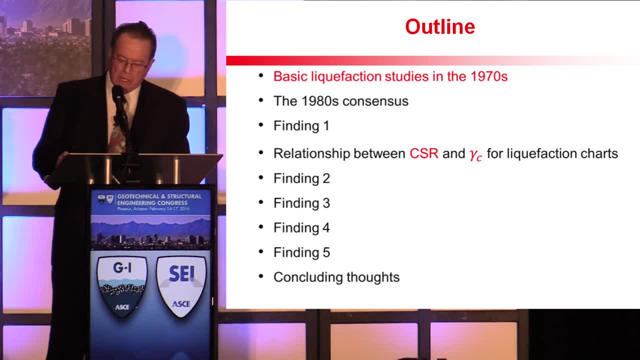 This is the outline of the rest of the talk. I will start with a review of some key liquefaction issues in the 1970s. That shows you how old I am. I mean I was reading papers. I think I made about four papers at the time. 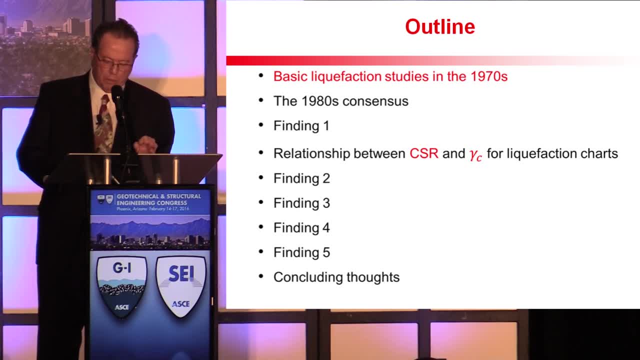 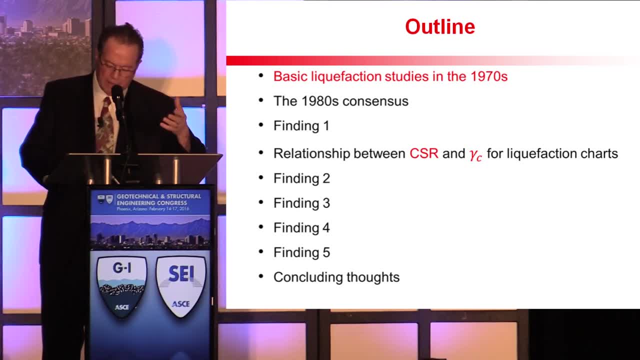 and the cyclic shear strain which we saw earlier, gamma sub C, which is an alternative parameter to CSR. that also describes in a different way the demand imposed by the earthquake on the soil. Let me say a couple of things first about the basic liquefaction studies in the 1970s. 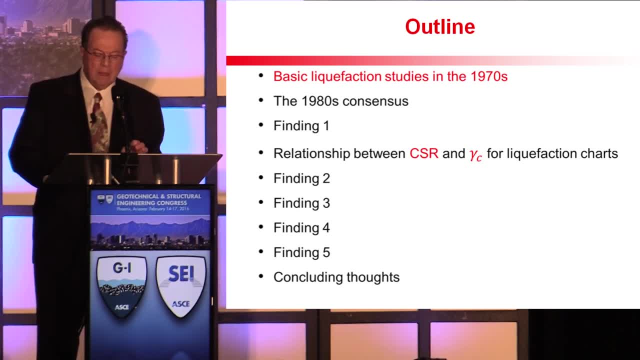 before I move to the next slide, The main breakthrough was a model developed by Martin Finn and Seed that related densification of a sand subjected to cyclic shear loading in drain condition to the increasing pore pressure in the same sand due to undrained. 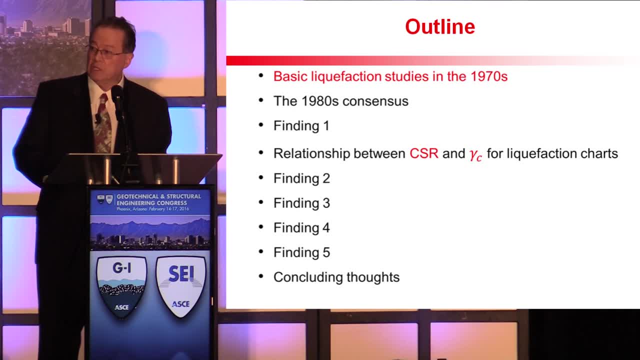 cyclic loading. I don't have time to get into the details of this model. Let me only say that the model was verified by several laboratory studies in the 70s and 80s And, very importantly from my viewpoint, point today. it told us that the best way to understand 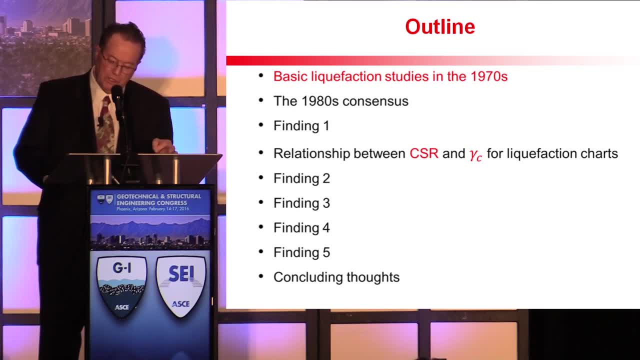 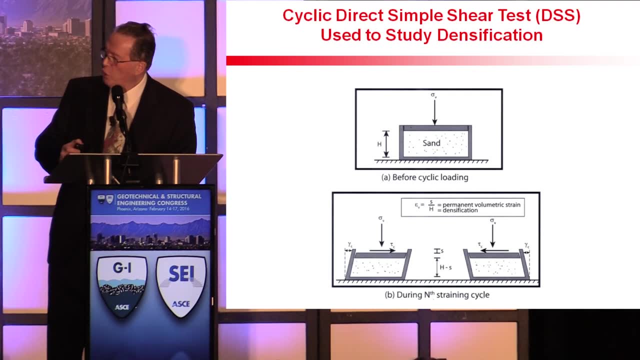 the PoI build up at the basic level is to look first at what happens to the densification of dry sand subjected to cyclic loading. So let's look at densification of dry sand subjected to cyclic shear. An excellent study of this was done also in the 1970s by Silver and Seed at the University of California. 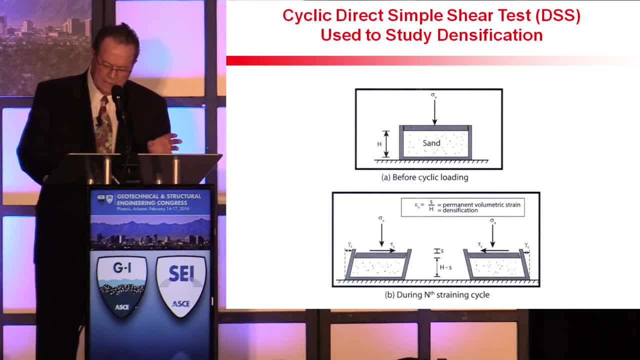 Berkeley. They used a device which was not quite identical to the direct simple shear sketching model but to check for any change in the density of the sand particles at the bottom of the sand. The standard temperature of sand was about 75 degrees and the density 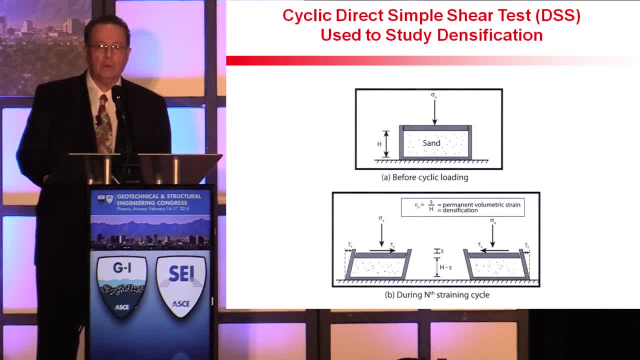 of the sand was about 30 degrees And the average density was not necessarily the same in the 70s and 80s, but in the 90s the average density was almost 50 degrees And there were a couple on the screen but which provided similar boundary conditions. 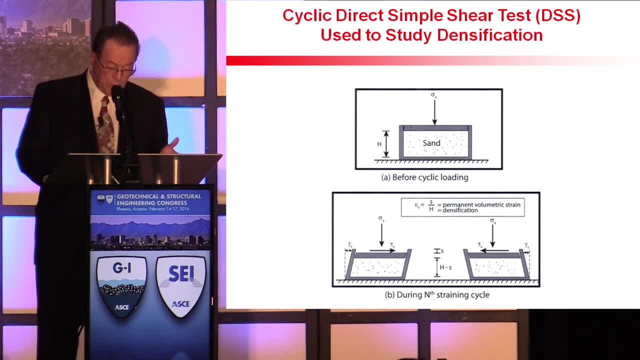 As you can see, what we have is essentially a consolidometer with rigid walls used to compress the dry sand under the vertical pressure sigma sub V, Except that the rigid walls are hinged at the bottom so that they can also rotate back and forth in order to apply cyclic shear loading. 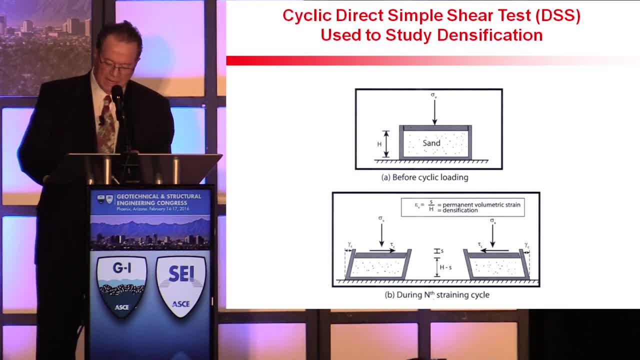 under constant sigma sub V. The cyclic loading that can be quantified either by the applied cyclic shear stress, tau sub C, that I would love to show you if I could, or associated cyclic shear strain, gamma sub C, produces in turn the sand densification. 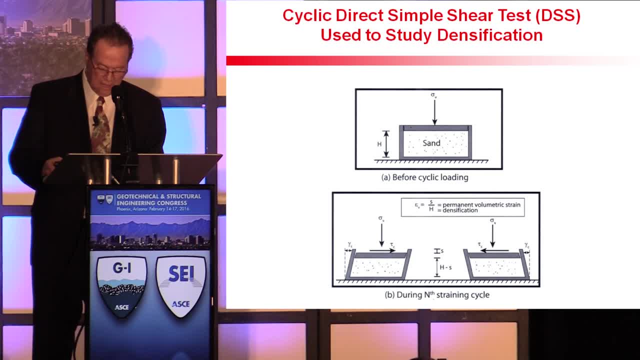 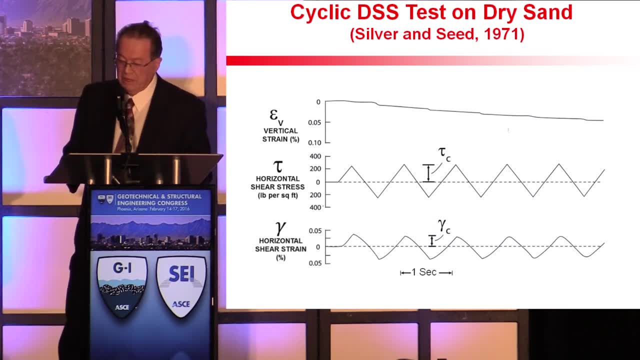 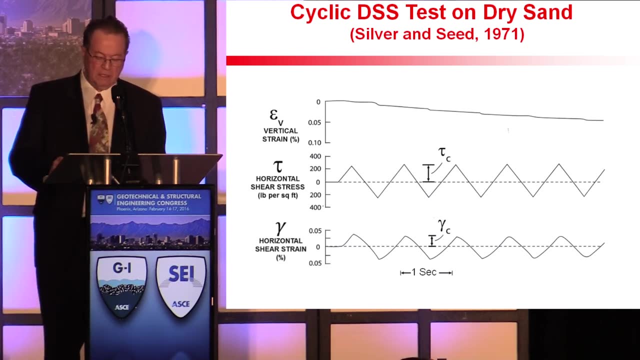 measured by the settlement of the top S and permanent vertical strain epsilon sub V. And here you have the actual traces of the dry sand under constant sigma sub V, measured in the first few cycles of one of the tests conducted by Silver and Seed with the shear loading applied at constant vertical pressure. 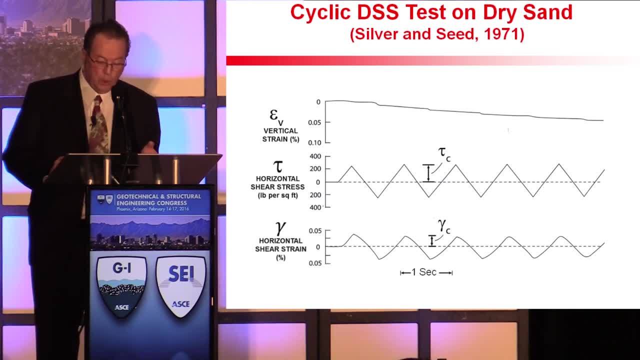 A constant cyclic shear stress was applied- tau sub C- which generated also a constant cyclic shear strain, gamma sub C, as there was no stress strain degradation. Therefore, these experiments can be interpreted as being either stress controlled or stress-controlled. So let's look at the test. 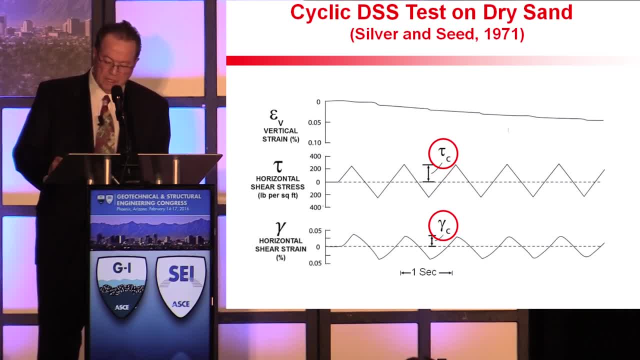 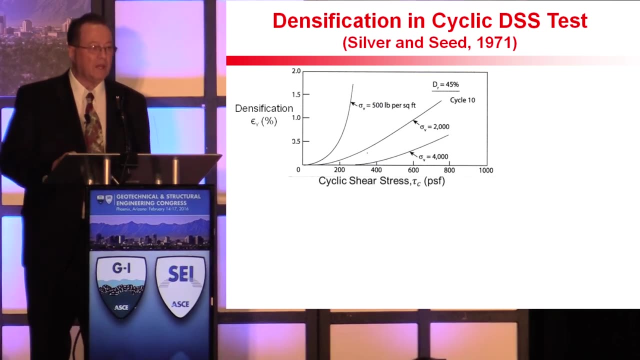 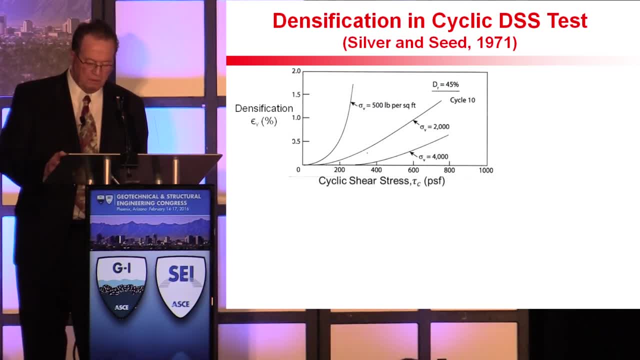 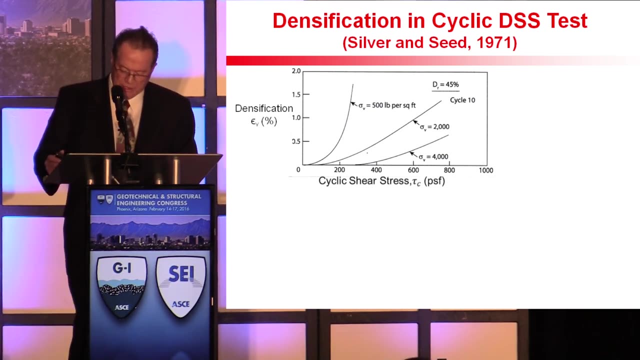 from several tests. The data correspond to densification measured after 10 cycles of a given tau sub C. The densification increases when the cyclic shear stress, tau sub c, increases. no surprise here. and for a given cyclic stress, densification decreases when the sigma v of the test is greater. But the most 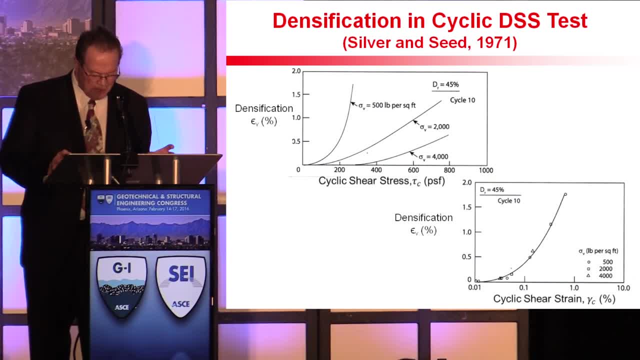 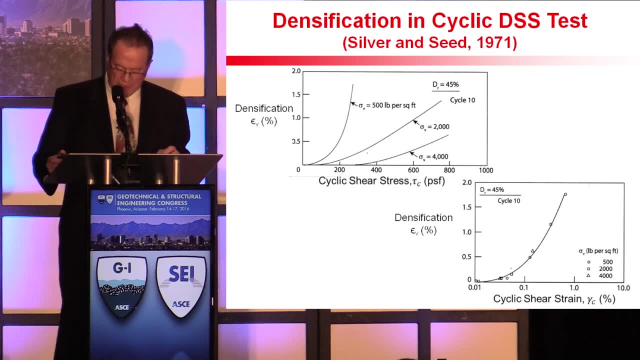 interesting plot is this one where the same densification is plotted instead versus the cyclic shear strain of the test. As you can see in this plot, the results collapse into a single curve which is independent of confining pressure. That is Silver, and Seed discovered that densification after a 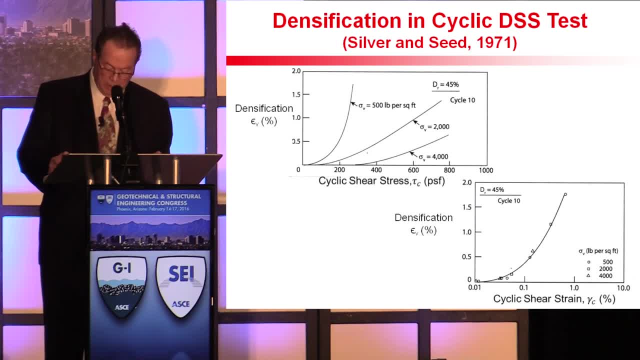 given number of cycles, given sand, relative density, etc. is independent of effective confining pressure and therefore of depth in the field if the cyclic shear strain is used as parameter instead of the cyclic shear stress. On the basis of this finding on densification, 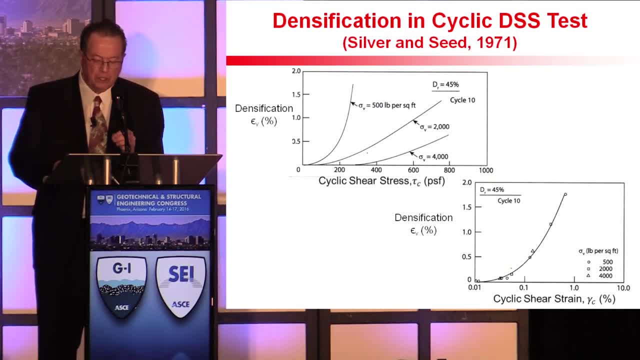 the result is that, together with a close relation between densification and pressure buildup found by Martin Finn and Seed, a group of us that at the time included also Richard Ladd, Jen Stokke and Les Joud proposed to use cyclic shear. 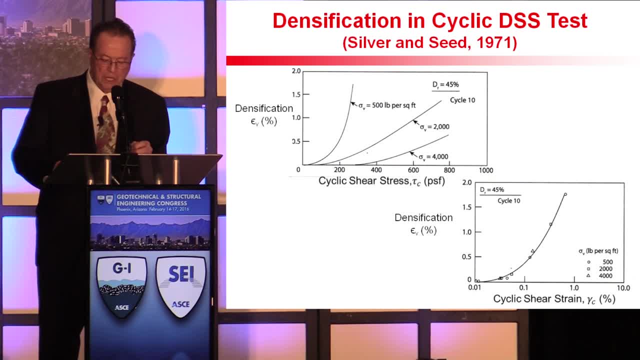 strain instead of CSR as a basis for a new generation of liquefaction charts for field evaluation of liquefaction potential. Between other things, this would have brought into the picture of the shear wave velocity, which is a measure of the shear stiffness of the soil. It was quite a 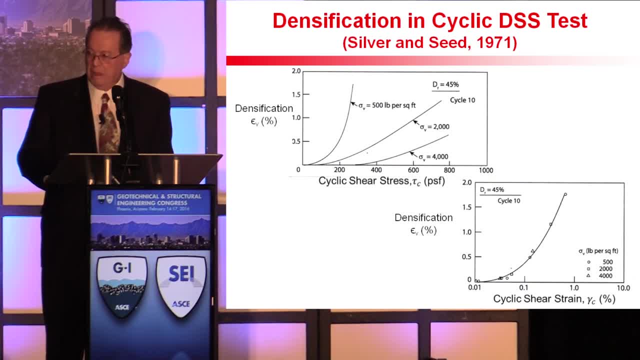 radical proposal and also premature for the tools available at the time. But hey, why not? We're all young and ready to change the world. The important thing from the viewpoint of my lecture today is that, as a result of that discussion, a 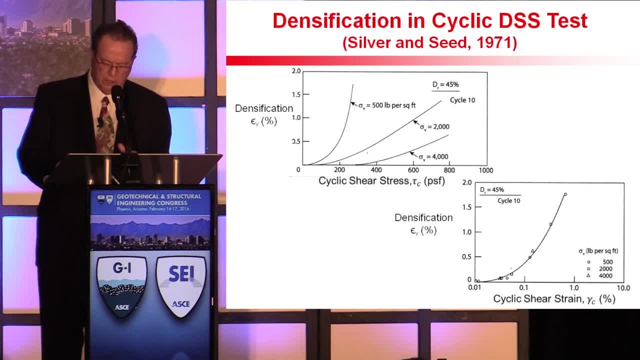 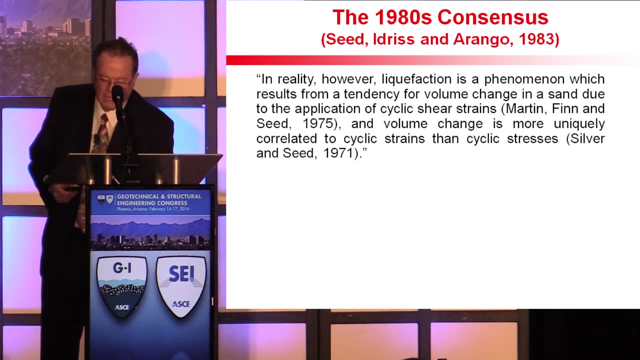 consensus developed which was beautifully summarized in a statement included in a paper by Seed Idriss and Arango. I have labeled this statement the consensus of the eighties, which in my opinion, is still completely valid today. Let me read the complete statement Quote: 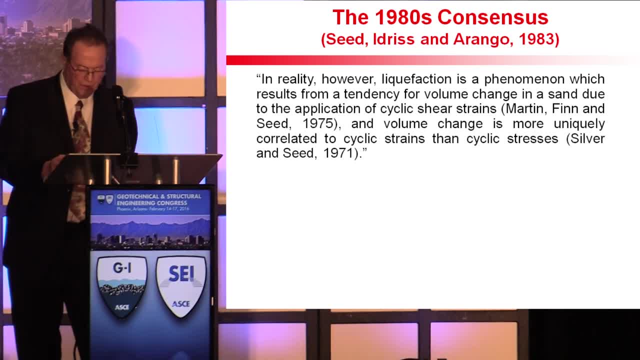 In reality, however, liquefaction is a phenomenon which results from a tendency for volume change in a. Let me read the complete statement. In reality, however, liquefaction is a phenomenon which results from a tendency for volume change in a Nessun due to the application of cyclic shear strains and volume changes. 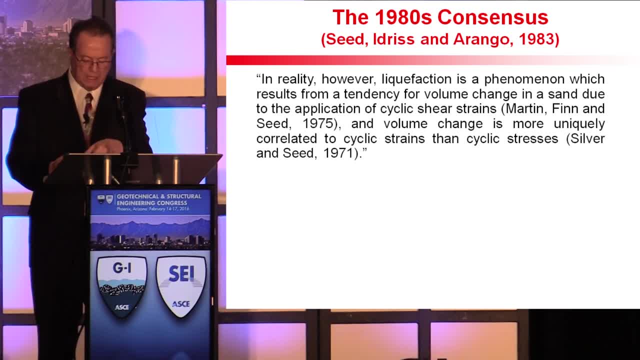 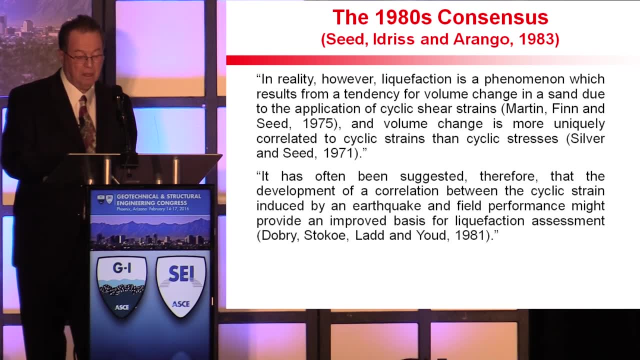 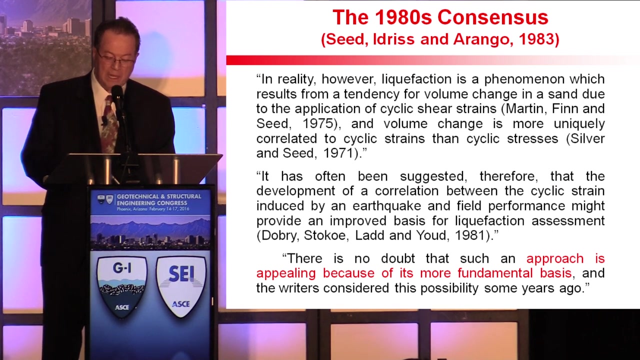 are more uniquely correlated to cyclic strains than cyclic stresses, Silver and Seed. It has often been suggested, therefore, that the development of a correlation between the cyclic strain induced by an earthquake and field performance might provide an improved basis for liquefaction assessment. assessment: Dobry, Stokke, Ladd and Yowl, 1981, the four young musketeers there. 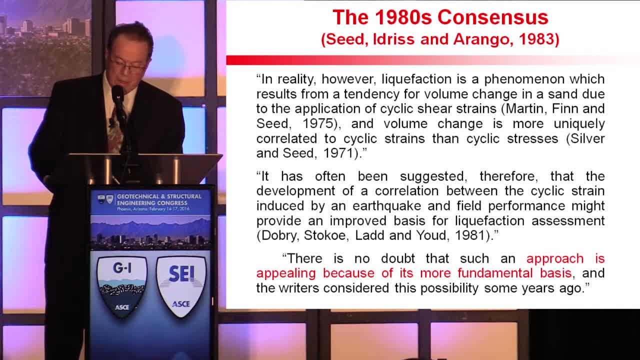 There is no doubt that such an approach is appealing because of its more fundamental basis, and the writers considered this possibility some years ago. end of quote. Now please note that by the 1980s, and as this quote says, Seed and Silver had demonstrated: 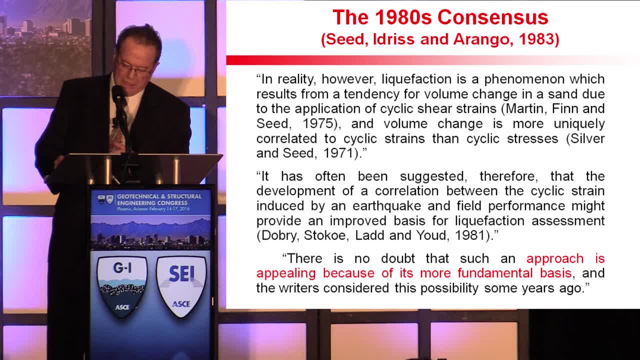 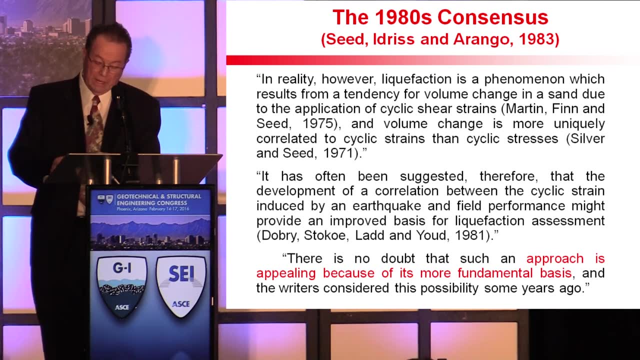 that densification is more uniquely related to cyclic shear strain than to cyclic shear stress. We assume that this was also true for pore pressure, but I am not quite sure this particular issue was completely settled at the time, But it was certainly settled, quite definitely. 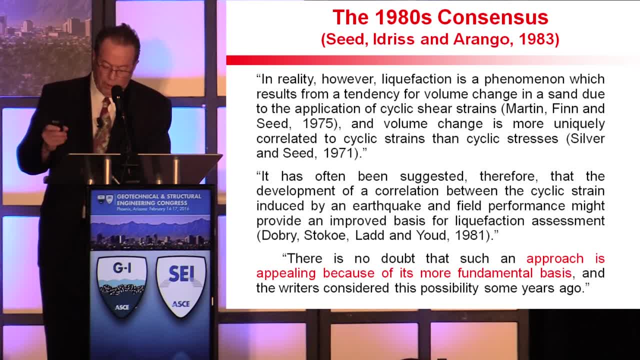 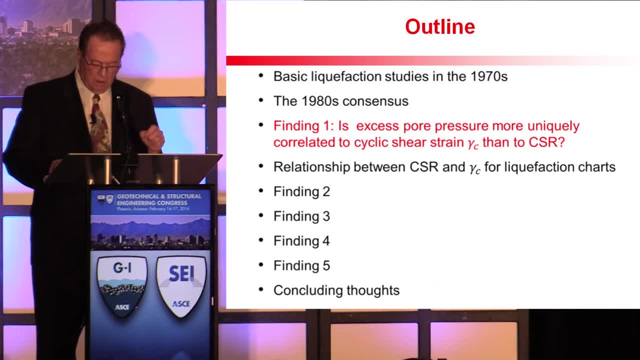 in my opinion a few years ago In one of our own projects, as I will show you in a minute, Which brings me to our finding number one. numero uno, Defined as the answer to the following question: Is excess pore pressure more uniquely related to cyclic shear strain than to cyclic stress ratio? 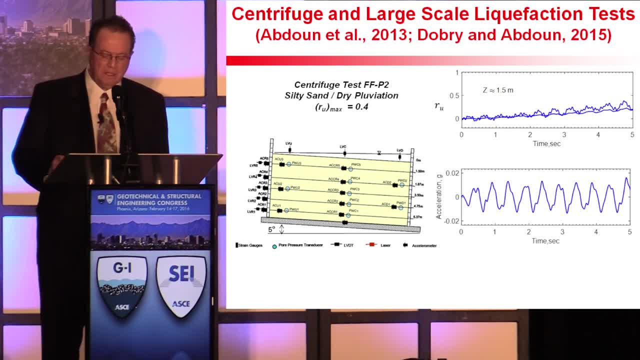 The answer to this question emerged from a series of studies that were done in the United States of four centrifuge tests and two large-scale tests conducted at RPI and at the University at Buffalo under the direction of Professors Abdoon and Tebana-Yagham. 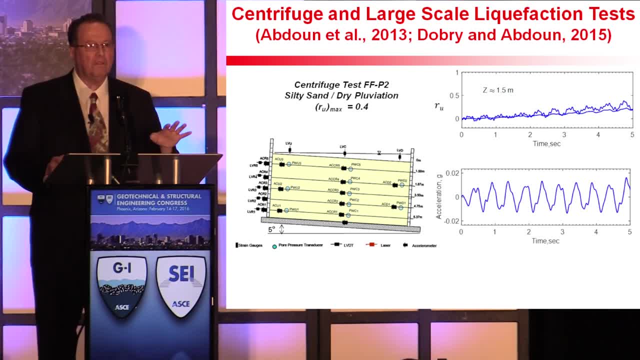 What you see on the screen is one of the four centrifuge tests conducted on a silty sand with 21% fines, having a relative density of 35% and placed as a uniform deposit six meters thick in the prototype. That's also one of the surprises of RS-10, since both Arizona 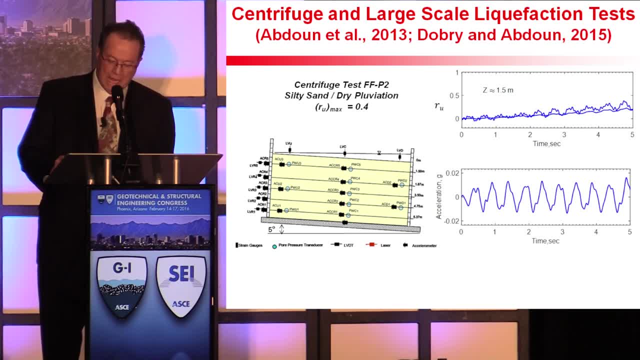 and West Virginia were tested for force pressure gain. The six deposits were tested including both inclined and level cases, and the inclination didn't make any difference in the pore pressure results. The model deposits were instrumented with piezometers, accelerometers and other sensors. 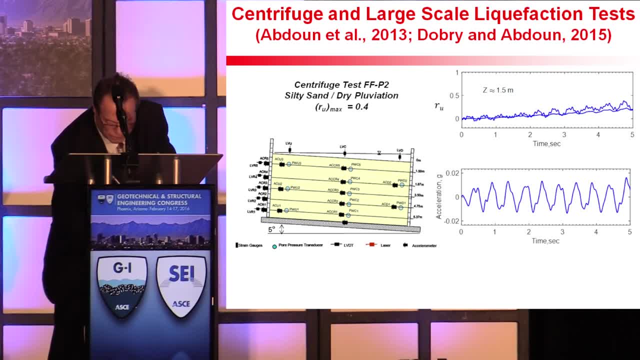 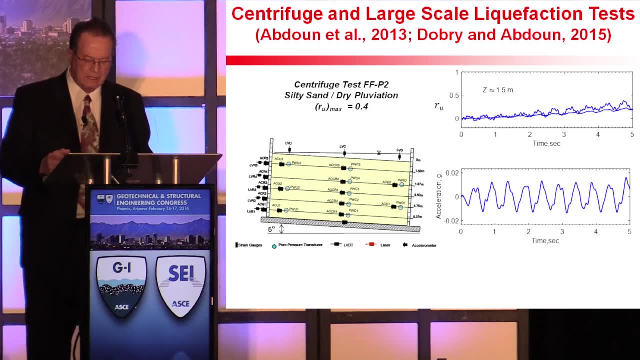 mostly embedded in the soil. The deposit was subjected to these 10 cycles of constant amplitude acceleration at the base. The peak base acceleration in this and the other tests was only about 0.02 g- small acceleration as the purpose was not to liquefy the soil but to generate enough excess pore pressure. 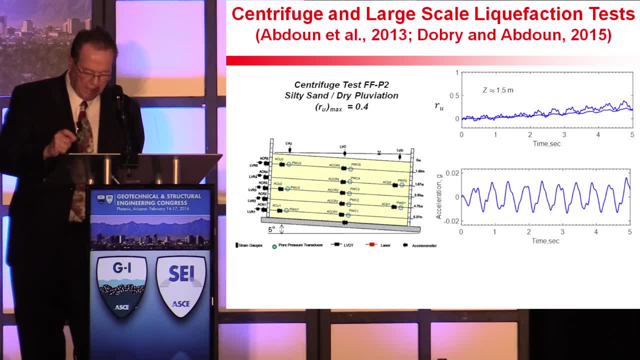 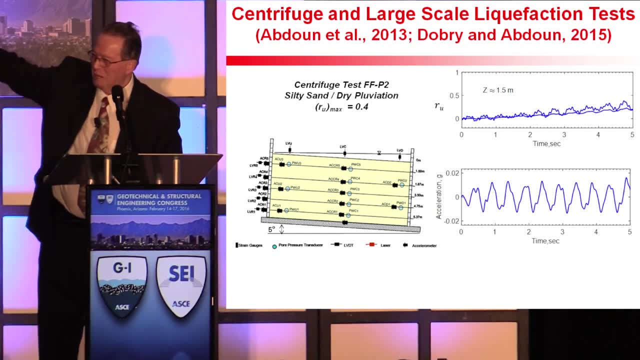 short of liquefaction, so we could start the pore pressure buildup as it approaches liquefaction. Here I'm pointing to it. right, You have the excess pore pressure ratio recorded in this test by the shallow piezometers, where the pore pressure ratios were greatest, which by the end of shaking had reached a pore pressure. 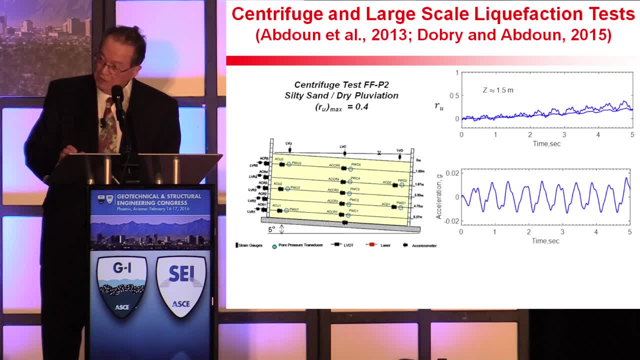 ratio of about 0.4, significant but still far from liquefaction triggering. that would occur at a pore pressure ratio of 1.0.. All six days, The deposits of loose sand had the same prototype thickness of about six meters. They were all subjected to the same base acceleration. 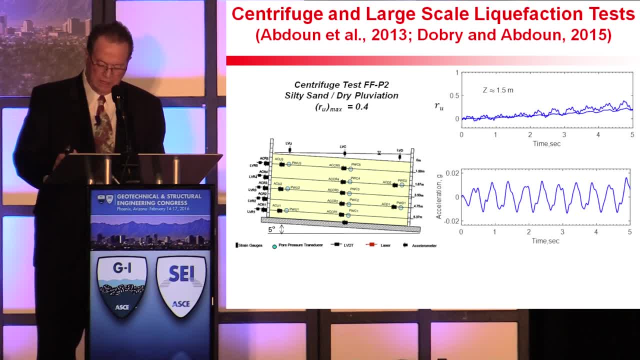 But there were also two differences. One, some tests were done with the silty sand and the others with clean sand, And two, we used dry pluviation in some of the tests and hydraulic filling in the others, therefore creating two different types of soil fabric, with soil fabric influencing significantly. 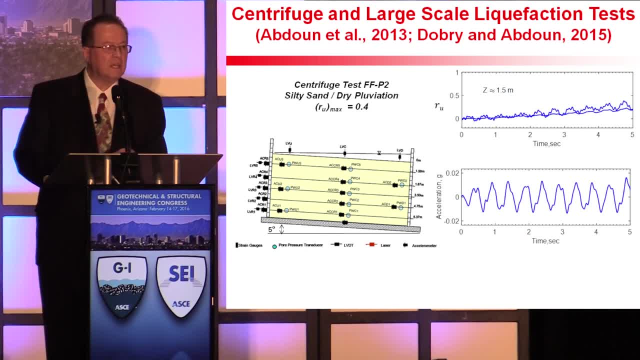 the results. So it was the same prototype thickness of about 6 meters And the same prototype thickness of about 6 meters. results: By covering this range of sands and soil fabrics, we started approaching the diversity of conditions we find in the field, Because the pore pressure 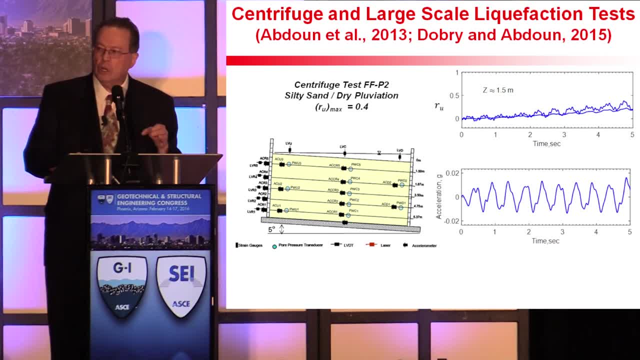 buildup was limited in the six tests. there was not much stress strain degradation So we could process the horizontal acceleration records at different depths using system identification To extract the shear stress time history tau at mid depths in the deposit, which is this trace here. 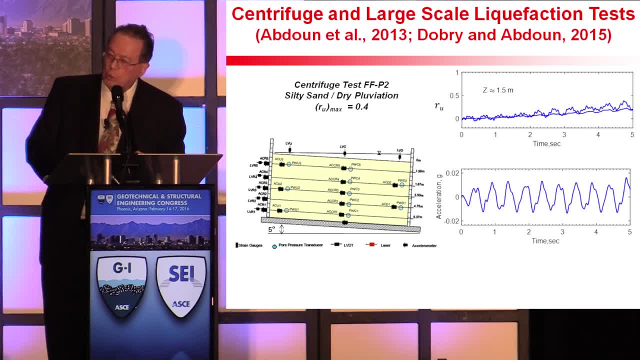 with a peak shear stress of about 2 kPa. Similarly, we could extract the shear strain gamma at the same depth, which is this other trace here, with a peak shear strain of 0.03 percent or 0.04 percent, As you can see in the two traces there is. 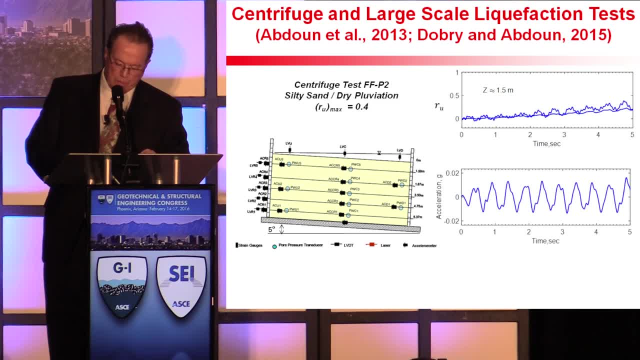 essentially no stress strain degradation, Except perhaps a a little bit near the end of the time history of gamma, where there is some starting. Therefore, this centrifuge experiment can be considered either as a test of constant cyclic shear stress, tau sub c, or constant cyclic strain gamma sub c. 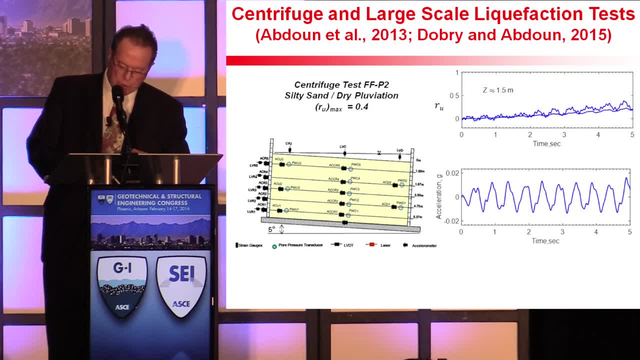 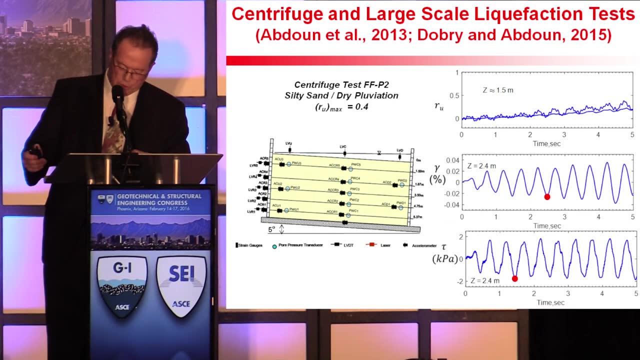 where this single value of stress or strain can be used to represent the whole time history, We selected gamma sub c and tau sub c as the median of all 20 peaks or so in the corresponding time history. Here you can see the peak selected for gamma sub c. 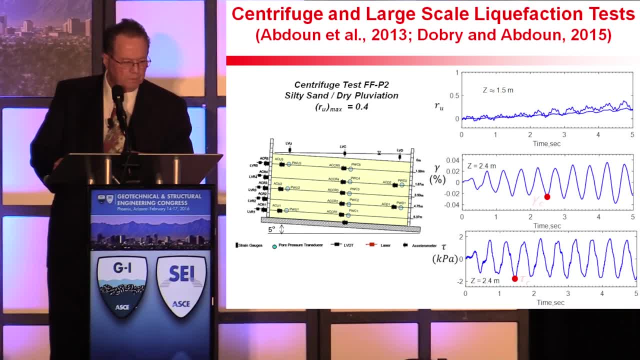 and here is the peak selected for tau sub c. These two selected values of gamma c and tau sub c correspond to different peaks. With the method we used, there was no reason for them to happen in the same peak and it doesn't make too much difference anyway. 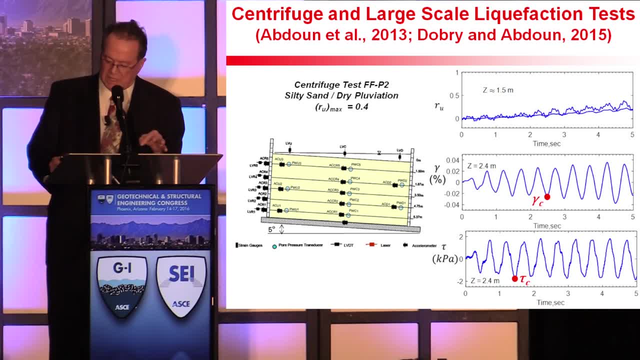 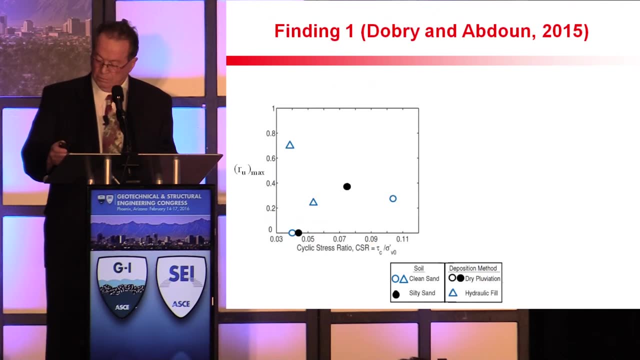 Finally, we obtained from this selected tau sub c the value of the cyclic stress ratio, or CSR, of the test by just dividing it by the effective vertical pressure at that depth, And here you have the first graph where we plotted the maximum pore pressure ratio, Ru max. 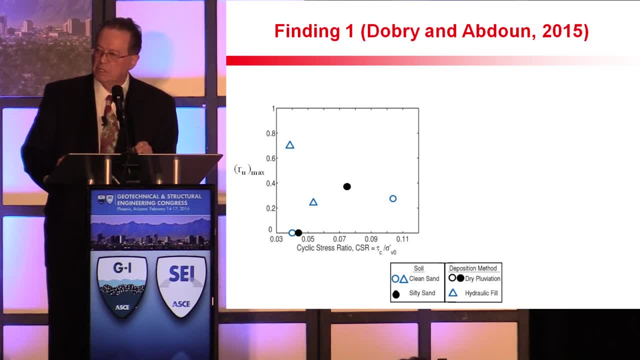 measured in each of the six tests, these six data points, or one test each, versus the cyclic stress ratio of the test CSR. The plot does not show any particular correlation between the two parameters. And here you have the corresponding plot for the same Ru max. 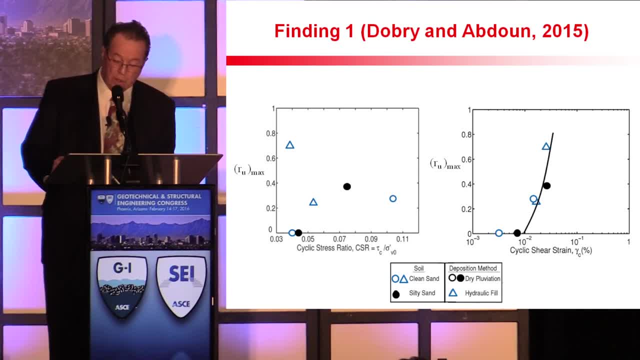 but plotted now versus the cyclic strain of the test, where the correlation is much better. In fact it's quite good. We find here for pore pressures the same thing as for the cyclic strain of the test. the same thing: Silver and Seed found. 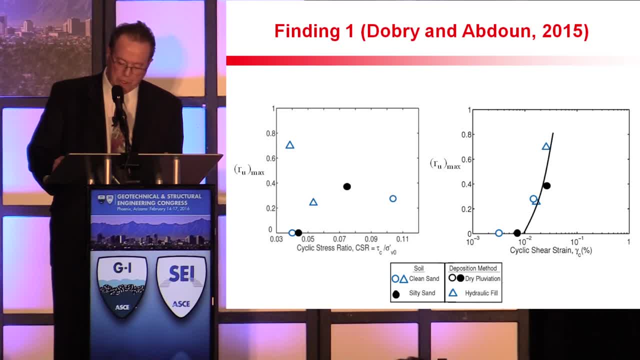 for densification of dry sand that the pore pressure is much better correlated to cyclic shear strain than to cyclic stress ratio. Let's focus on the plot on the right For the two tests which had a gamma sub c less than the threshold strain at about 10 to the minus 2%. there are two data points there which show no pore pressure buildup at all in the sand, as expected, While above the threshold, there is a fast increase in Ru max as gamma sub c increases, with values of pore pressure ratio between about 0.4 and 0.7 at a strain of about 0.025%. 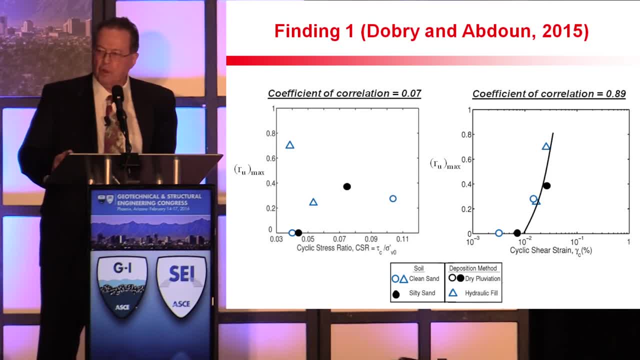 We also computed for the two plots the coefficient of correlation, usually called R in the statistical literature, And as you can see, it is 0.89, close to 1.0.. Corresponding to perfect correlation for the strain plot, And only 0.07, close to 0,. 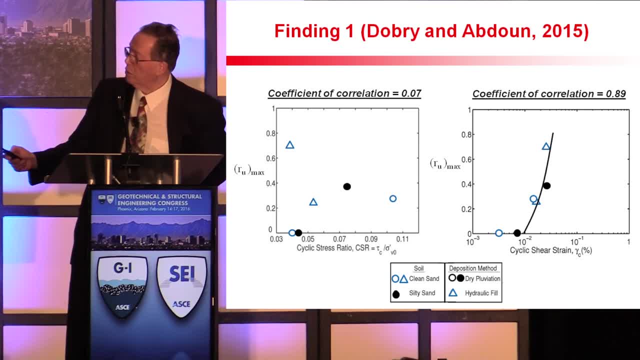 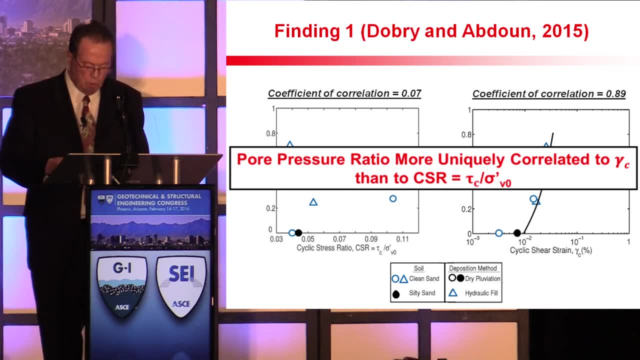 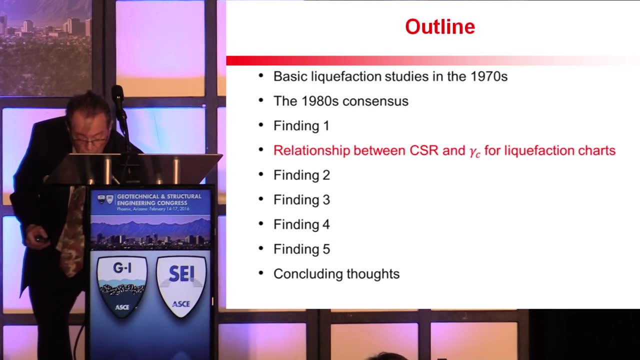 corresponding to no correlation for the CSR plot. Therefore, here is our finding number one: Pore pressure ratio is more uniquely correlated to gamma sub c than to CSR. The next step is to find the correlation between gamma sub c and 0.025.. 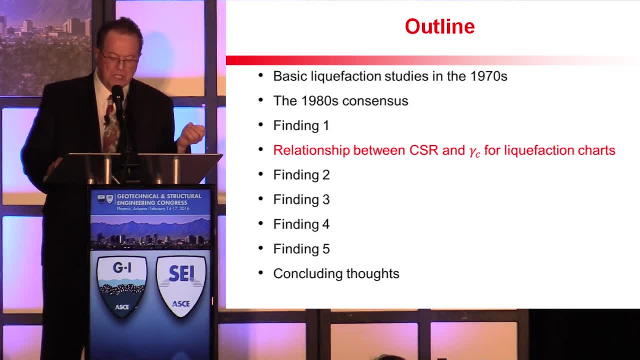 The next step is clearly to investigate what is the level of cyclic shear strain gamma sub c associated with liquefaction in the field during actual earthquakes. We can do this by going to the liquefaction charts, which, after all, have been calibrated by field case history. 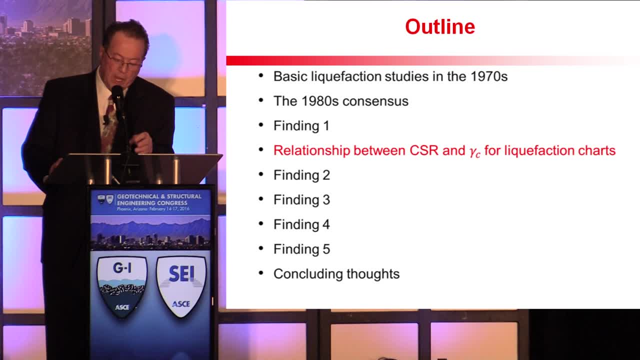 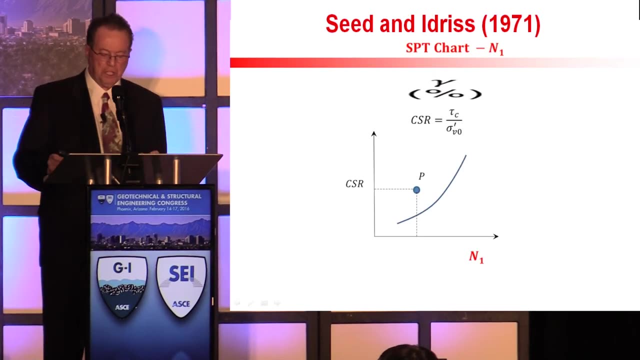 The charts, however, use CSR, So we first need to find an equation to calculate gamma sub c from CSR for any point of the chart. We will develop that equation in the next few slides. Okay, here we go. We have this liquefaction chart. 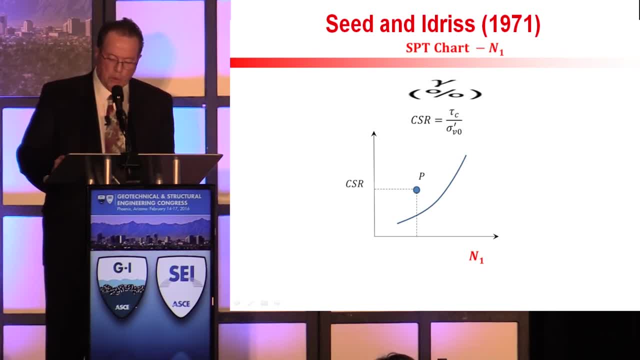 Let's say the original Seed and Ingress chart based on the SPT, And we want to know the value of the cyclic shear strain gamma sub c for this point P on the chart, for which we know two things: CSR and the normalized SPT, which is N1.. 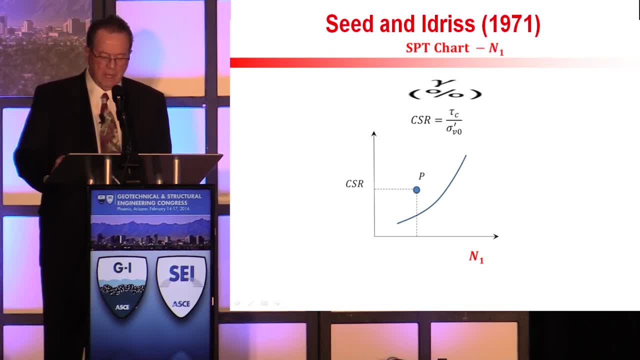 At the top are the two main definitions of CSR: the one mostly used by practicing engineers which use the peak ground acceleration A sub max, And the second, more basic definition, where CSR is defined as the ratio between the representative cyclic shear stress in the layer tau sub c normalized to the effective overburden pressure. 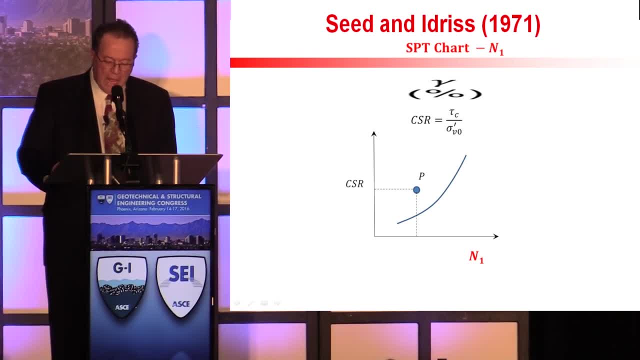 before the earthquake: sigma prime V0.. I am going to develop the equation between CSR and gamma sub c using an animation Which is nice. I mean, it's distracting, fun, like going to the movies. I will also go fast, But this should not be a problem. 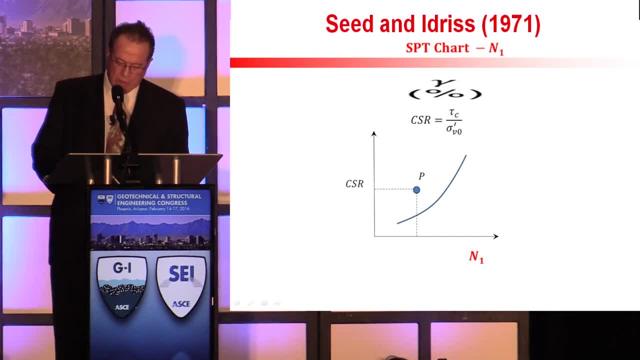 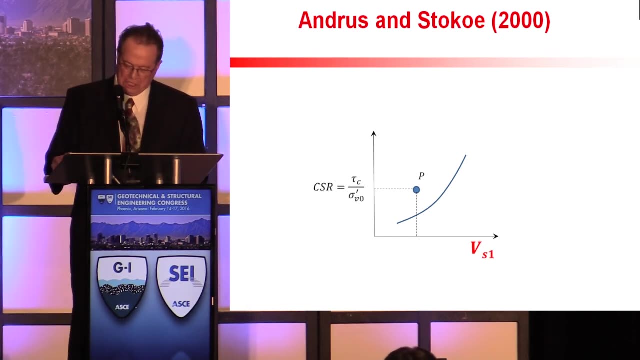 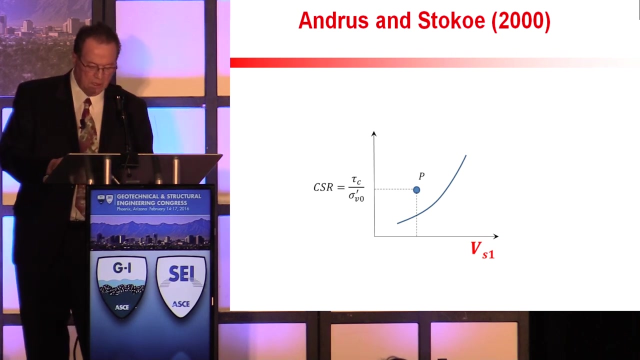 as most of you are very familiar with the plots, symbols and intermediate expressions I will be using. We just switched to a shear wave velocity chart Like, for example, that proposed by Andrews and Stokke, With VS1 at the bottom instead of N1. 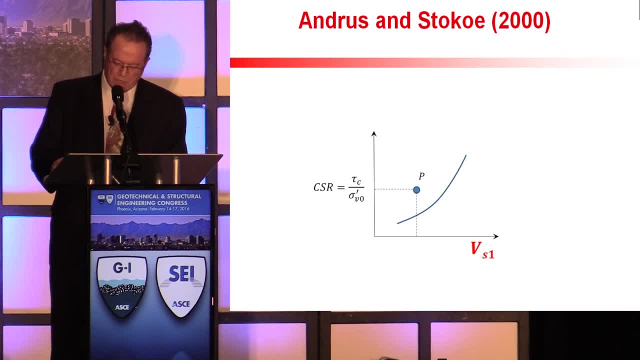 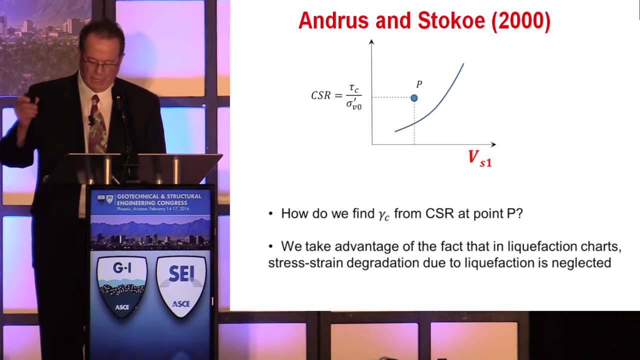 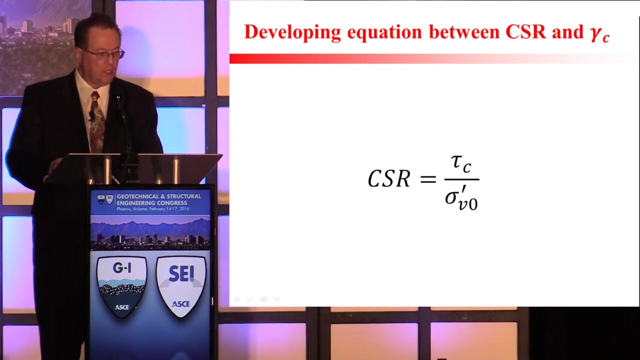 Can we do this? Of course we can If we have measurements of both SPT and VS at the side. Okay, This is our starting point. Let's now begin our derivation, where we will convert this definition of CSR into an equation relating CSR to gamma sub c. 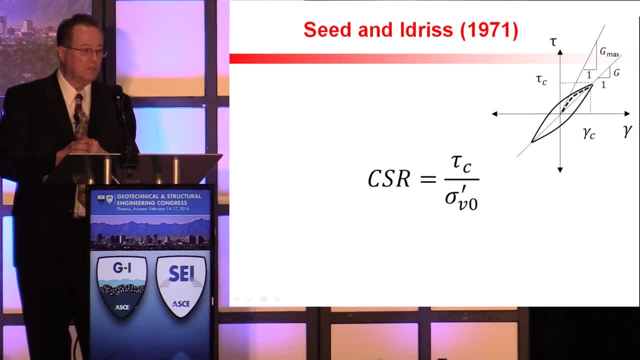 We go back to the classic hysteresis loop, which you have seen many times if you ever took a soil dynamics course, Where tau sub c and gamma sub c are defined as the coordinates of the tip of the hysteresis loop for cyclic shear loading of soils, including sands. 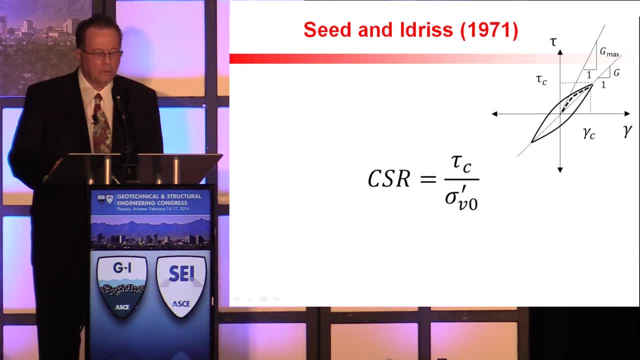 G is the secant shear modulus, which is tau sub c divided by gamma sub c, And g max is the value of g at very small strains. Therefore, this is true, And this is true, And therefore we can replace Nice, isn't it? 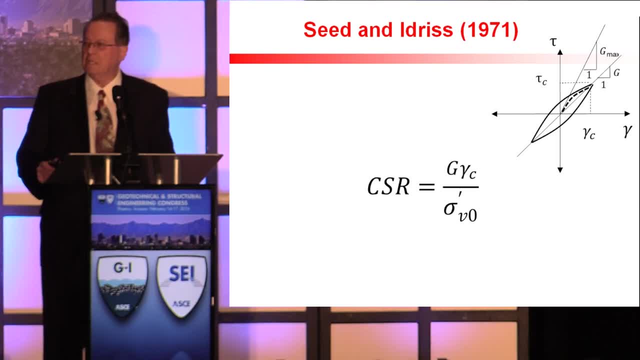 And gamma sub c has made its dramatic appearance. Its first appearance. But of course we have the g here which we don't know what to do with it. We have to transform it into VS somehow, And for that we need a couple of steps. 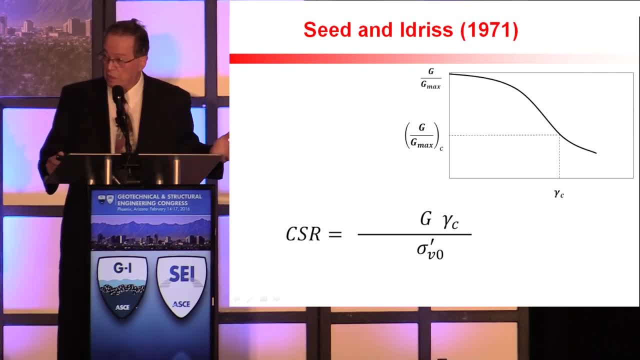 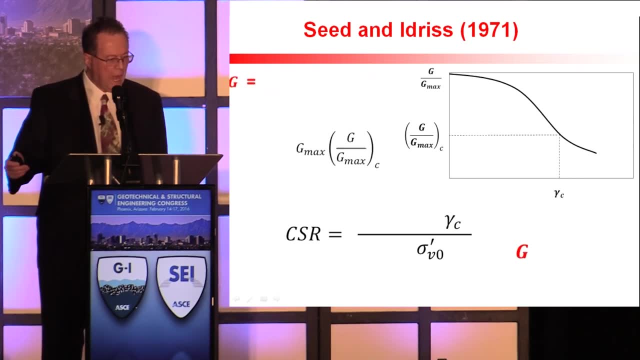 The first step is we go to the modulus reduction curve, Which you have seen many times, Which means that if we know gamma sub c, we know also g over g max And therefore this is true And we can replace: Okay, We have gamma sub c. 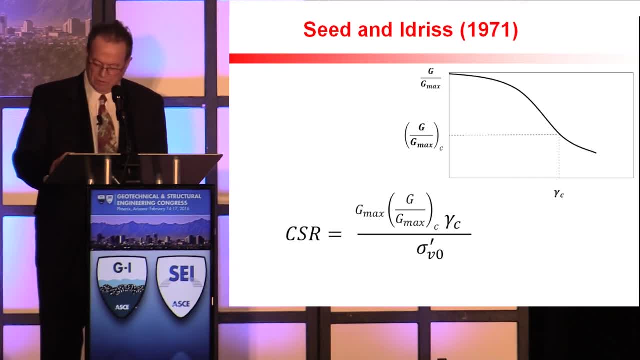 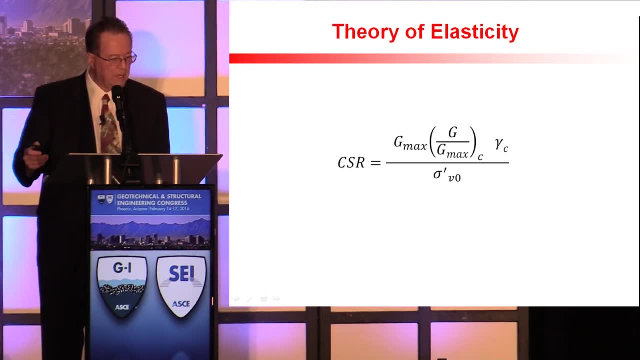 G over g max c, which is a function of gamma sub c, And we have g max And we have sigma prime v zero, which you should know for your site and layer And to replace gamma sub c for VS. we go back to theory of elasticity. 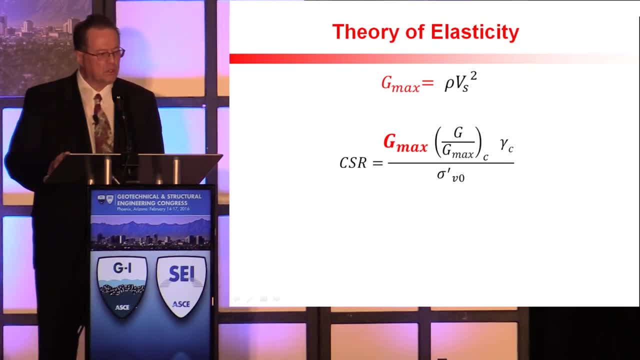 Under certain conditions. this is true. G max is rho VS square, Where rho is the mass density of the saturated sand, And therefore we replace- And we are almost there. All we have to do now is to replace VS by VS one. Its normalized version. 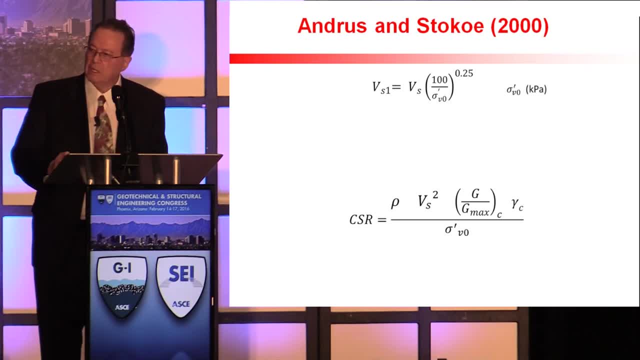 For which we go back to the definition That Andrews and Stokke provided for, that Sigma prime v zero is in kpa And therefore this is true, And we replace, And this is the equation, We simplify it a little bit. 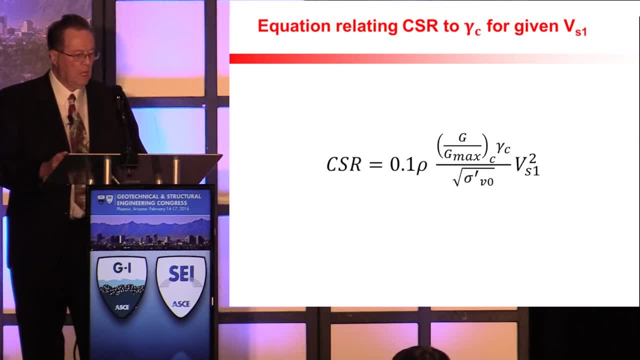 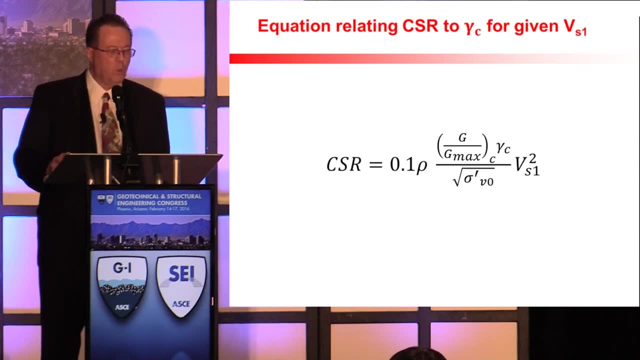 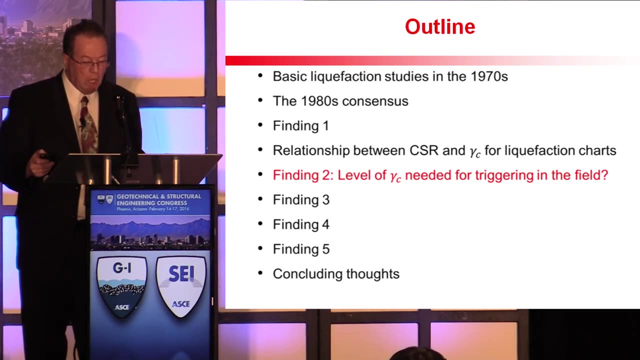 And we have this final version Where, if we know CSR and we know VS one And a couple of other things we should know- We can calculate gamma sub c. Armed with this equation- This is the equation- We can now go to the liquefaction chart. 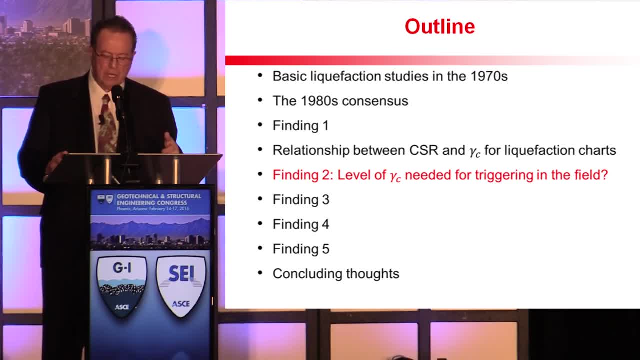 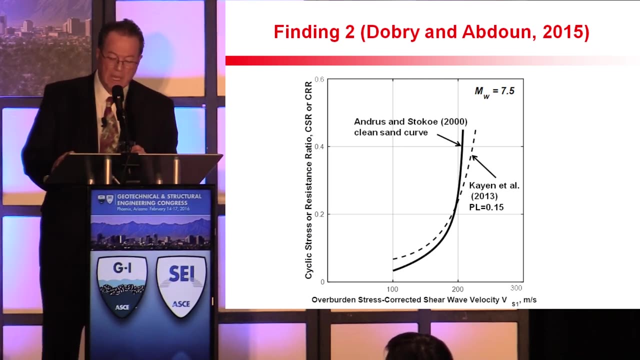 And find out what is the actual level of cyclic shear strain That is needed to trigger liquefaction in the field, As shown by the case histories in the field For which the charts are built. Here you have the same Andrews and Stokke. 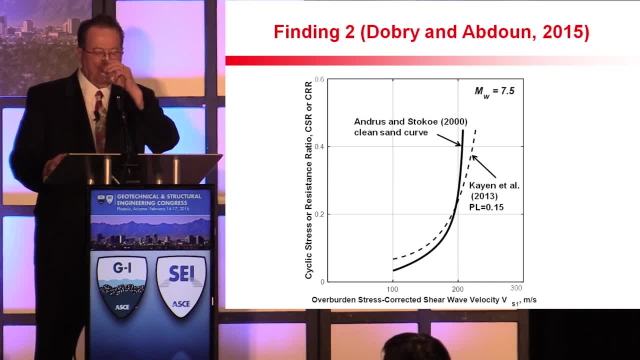 VS one chart you saw before, And I have also superimposed the more recent curve Proposed by Kayen and his co-workers. It gives the same results. Using the equation I just derived between CSR And gamma sub c, We computed the cyclic shear strain. 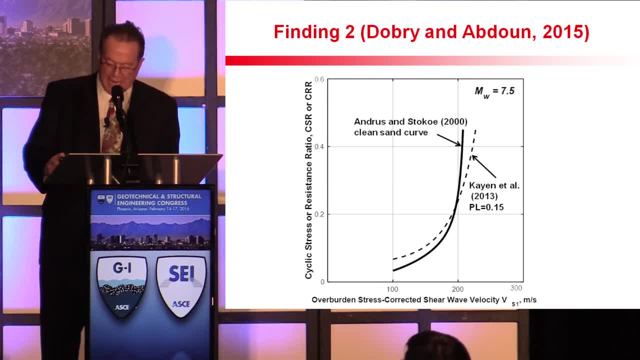 Needed to trigger liquefaction, Which we labeled gamma sub cl, At the two ends Of the Andrews and Stokke curve. We obtained the value Shown in red For gamma sub cl, About 0.03%, at the low end of the curve. 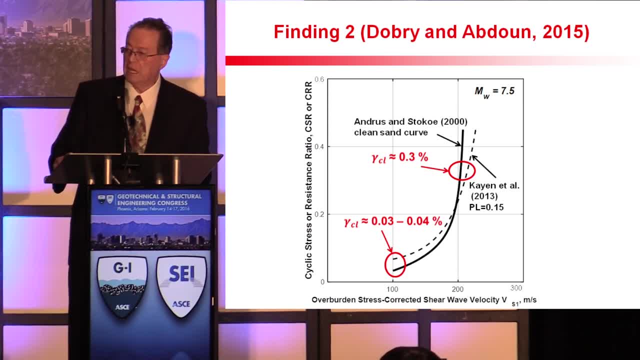 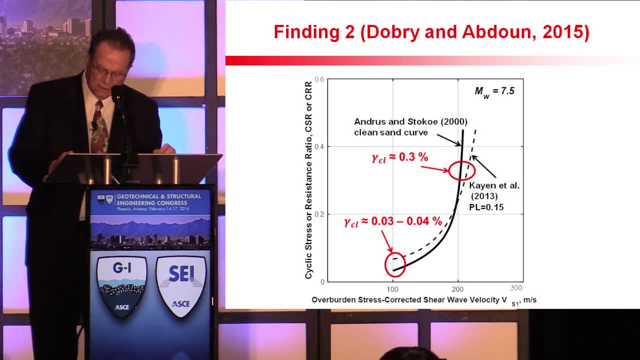 And 10 times higher, About 0.3% at the higher end. Let me add That Sid Idris and Arango, In the same 1983 paper I quoted before, Also estimated the gamma sub cl Corresponding to their SPT curve. 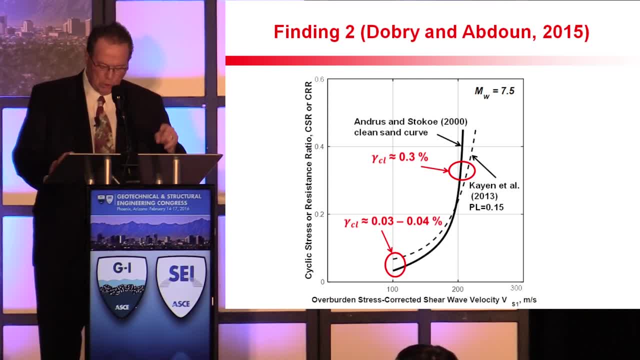 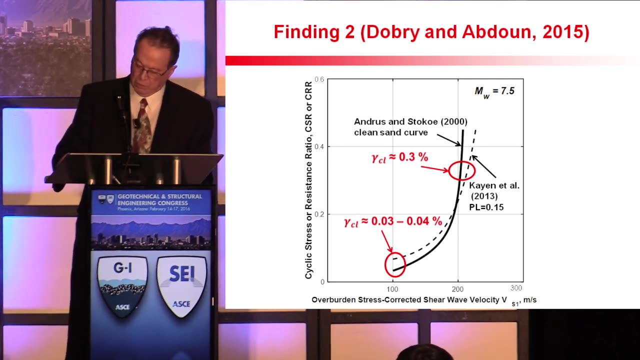 At the time Using a correlation Between SPT and VS, And arrive exactly to the same value Of 0.03%. we have here, Which I find A truly remarkable prediction Made 30 years ago. So Our finding number two: 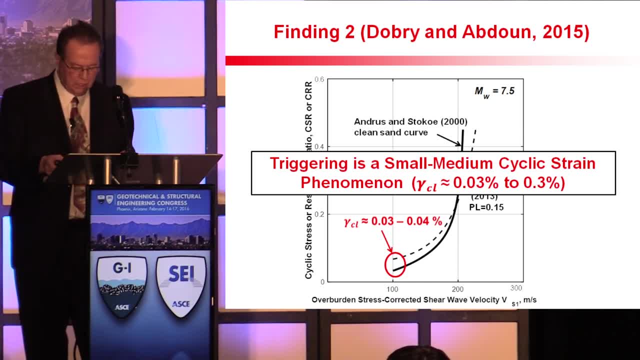 Is that triggering Of liquefaction in sands In the field During earthquakes Occurs at small to medium strains Ranging from about 0.03% To 0.3%. I think this finding Should be used by the profession. 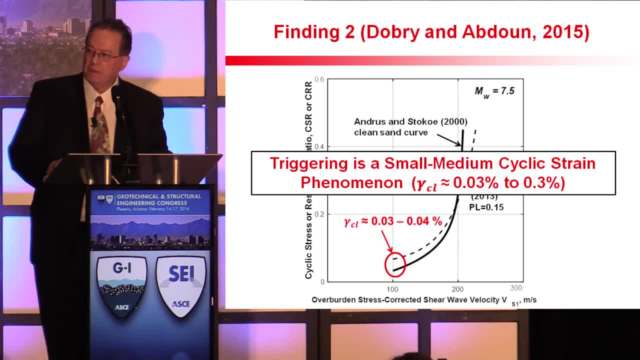 To reassess Some of the things We have been doing historically. So Does it make any sense To try to use critical state theory To understand triggering, When considering that critical state applies Only to much larger strains than this, Or should we still be using? 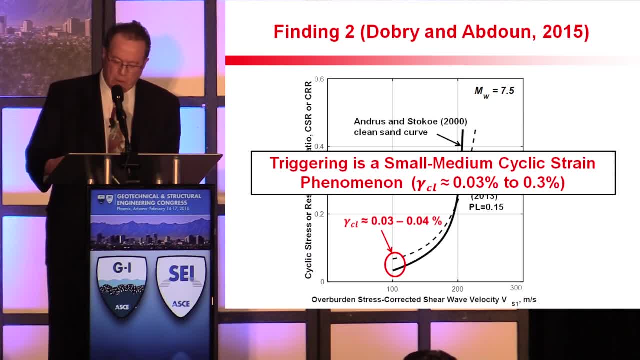 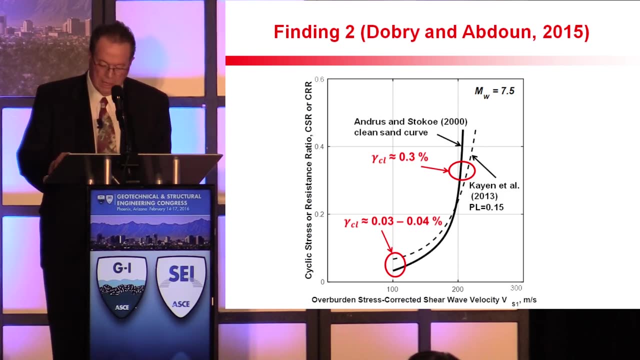 Result of stress control Cyclic triaxial tests For triggering evaluations, When the strains at the end of the test Sometimes reach 3% Or 4%, Too large to be relevant To the triggering phenomenon. Let me say one more thing. 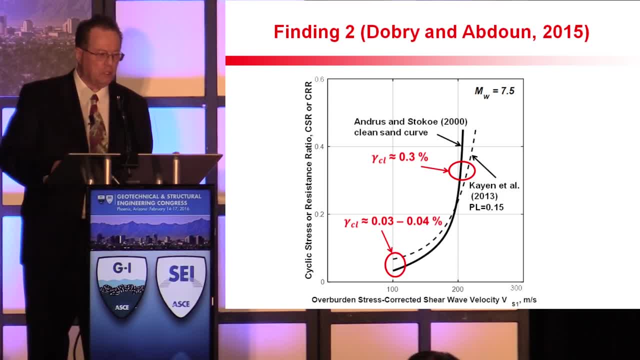 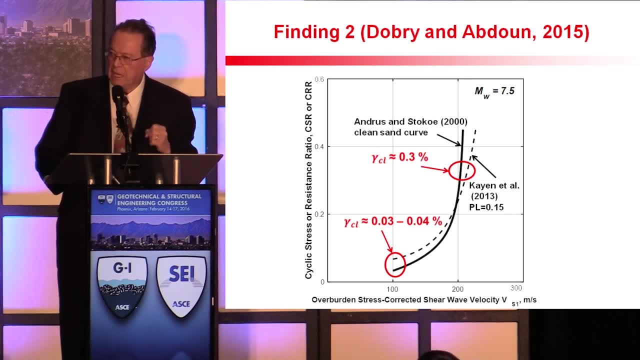 The lower branch of the liquefaction chart, Where we have the 0.03% Or so, Is known to be controlled By recent loose fields And natural sands. So We decided to explore the hypothesis That recent uncompacted artificial fields 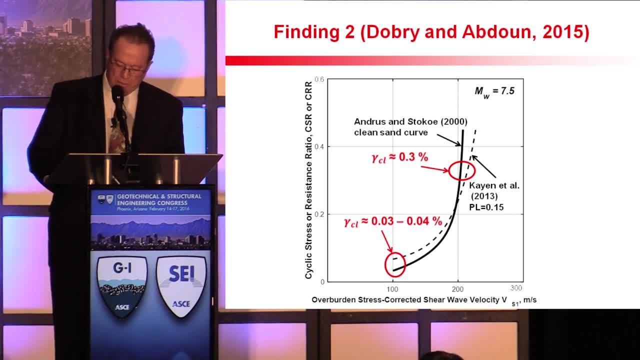 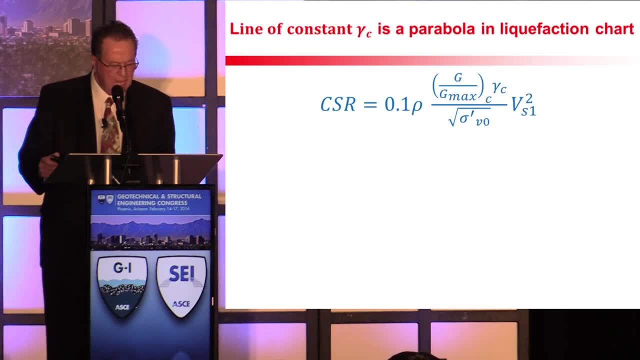 Have their own liquefaction chart Defined by a constant Gamma sub CL Of about 0.03%. But What is the shape Of this curve of constant triggering strain When plotted on a liquefaction chart? Well, Here is the same equation I derived before. 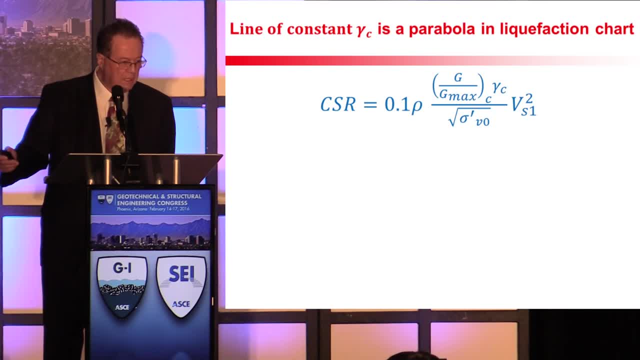 Between CSR and gamma sub C, Which can also be written In this other form As a function A Of gamma sub C Times VS1 squared, That is for constant gamma sub C. CSR increases With the square of VS1.. 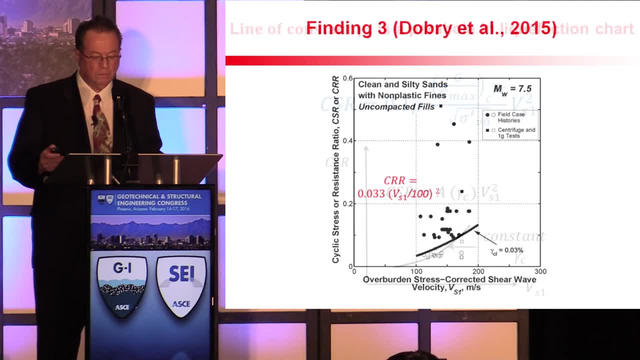 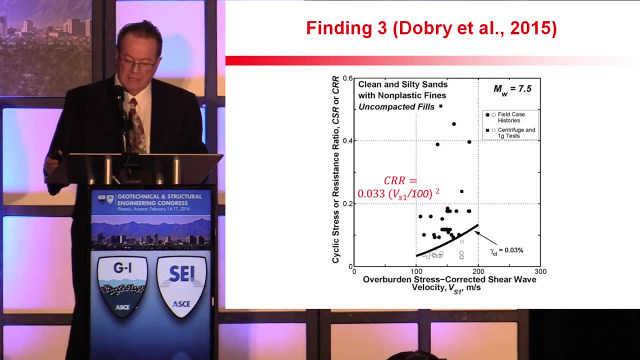 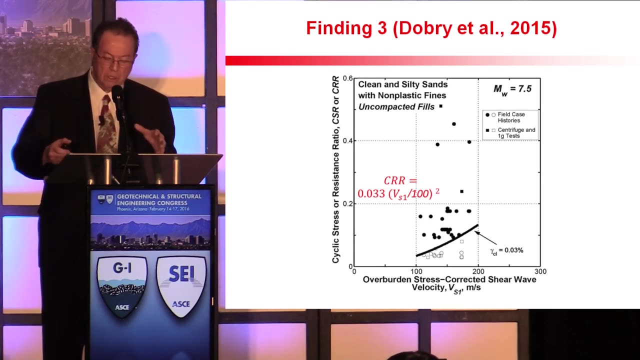 And the curve is a parabola. And this brings us To our finding number three. We took all case histories In the Andrews and Stokke database That were uncompacted Recent artificial fields And were also either clean sands. 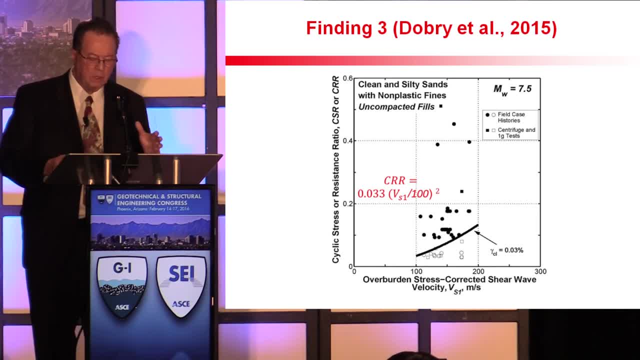 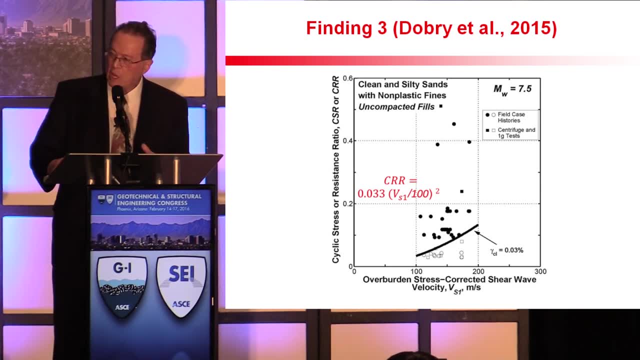 Or silty sands, up to 35% finds And we plotted them On the same chart of CSR Versus VS1.. For earthquake magnitude 7.5. We also included As additional case histories The centrifuge and large scale test. 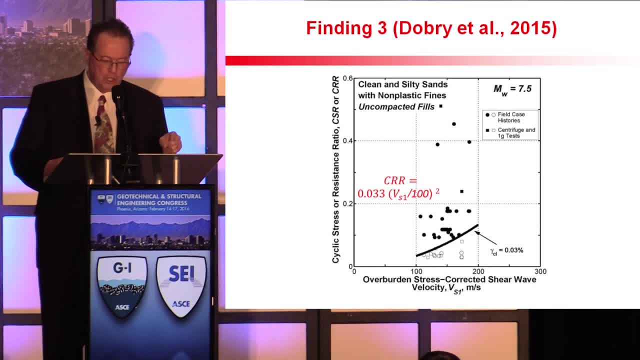 I showed you before And we were able to fit This constant strain parabola, Having the equation you see in red. CRR, Which is the value of CSR For points on the curve, Is equal to 0.033.. 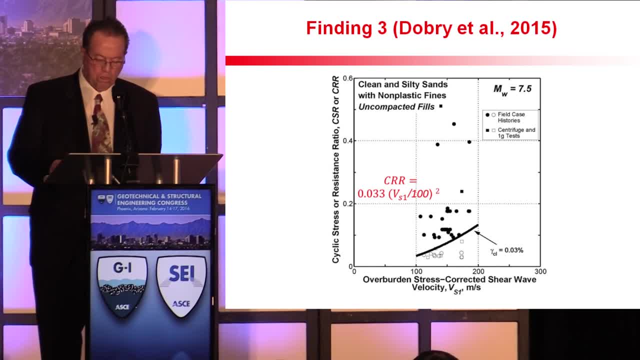 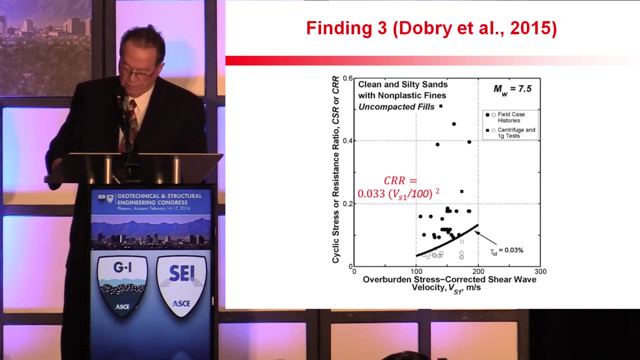 Times VS1 divided by 100.. All squared, You can see that this strain based curve Separates very nicely The cases of liquefaction From no liquefaction And corresponds, as expected, To a triggering cyclic strain Of 0.03%. 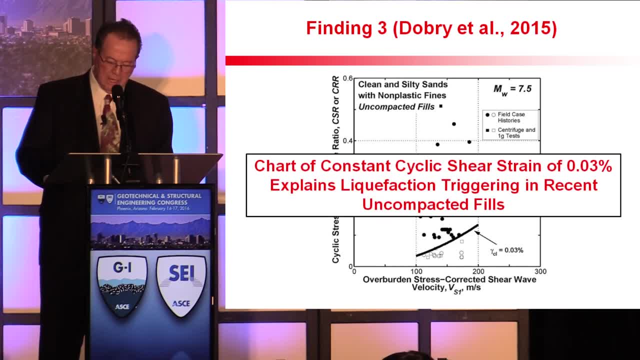 So Our finding three Is that liquefaction triggering Of recent uncompacted fields, With finds content Up to 35%, Is explained by a constant Cyclic shear strain curve, With the strain being 0.03% For an earthquake magnitude. 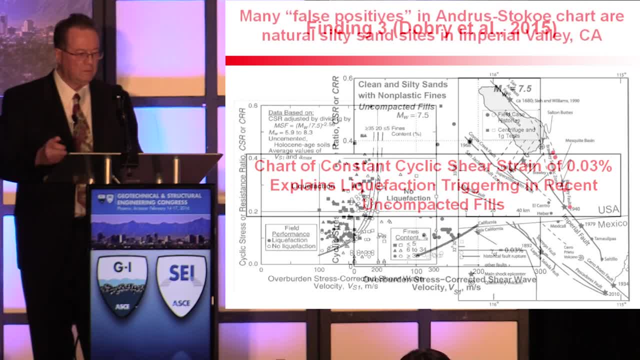 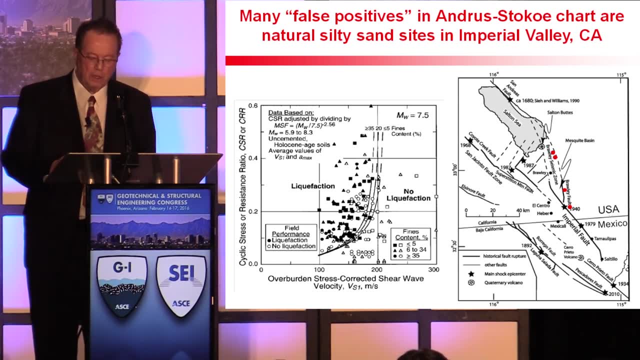 7.5. The plot thickens. Okay, Let's go back To the original Andrews and Stokke chart You saw before, Which you see again On the left. The data points in this chart Include a number. 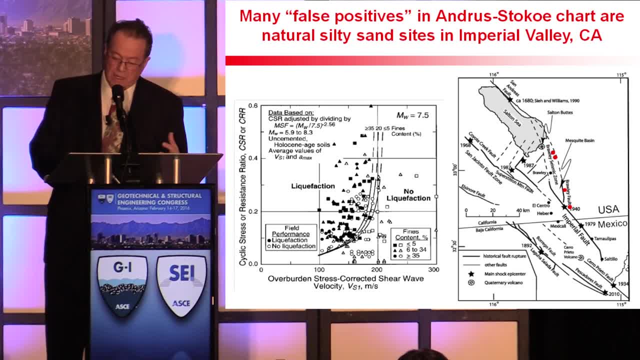 Of what have been called false positives. That is, size That should have liquefied Because they are above the curve, But in fact did not liquefy, And what we see here Inside this red oval, Are false positives. Well, 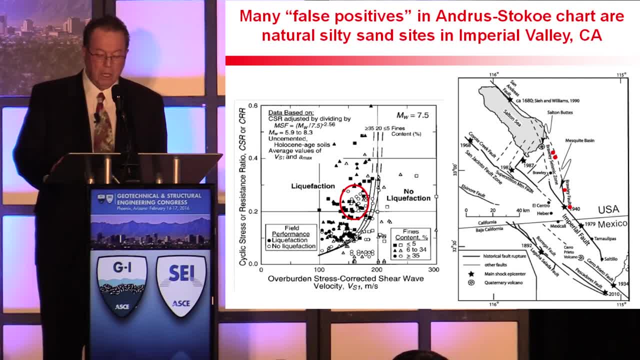 We found out that most of these false positives Are: They are not random data points. They are naturally deposited, Geologically young Silty sands located in a very specific Part of the world: The imperial valley of southern California. The map to the right. 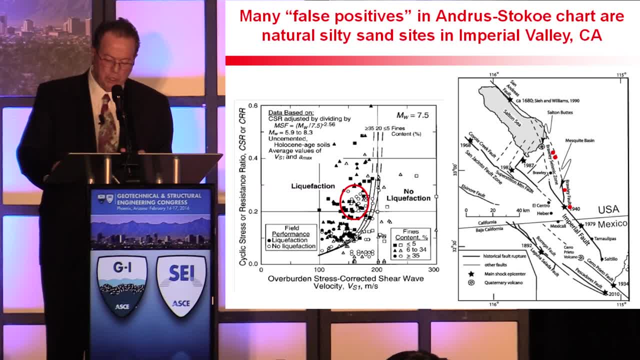 Shows the valley, And the four red dots Are sites Which provided all case histories In the Andrews and Stokke database. A main feature Of the imperial valley Is that there are a number Of active geologic faults And a lot of earthquakes. 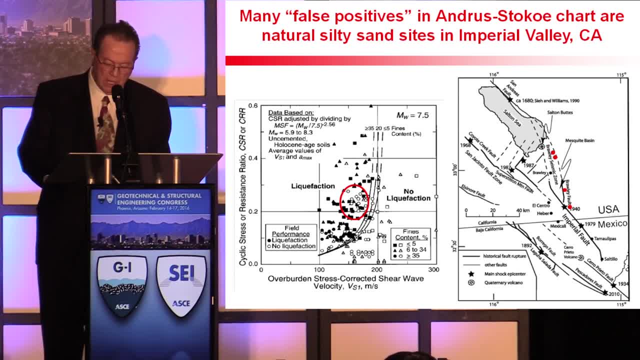 And this constant shaking Seems to be the main reason Why these sites have a higher Liquefaction resistance Than expected, Based on their values of VS1. And the Andrews and Stokke chart, For example, At one of these four sites. 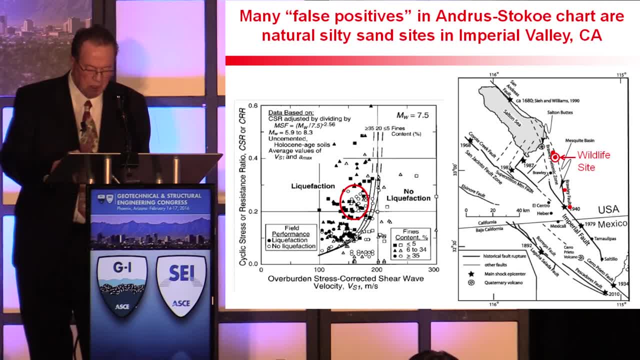 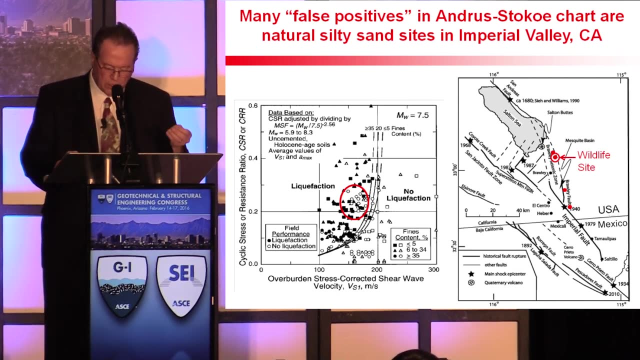 The liquefiable layer in the wildlife site I just named. That layer Seems to have been deposited In 1907. That is only a century ago, So It is younger That some of the artificial fields In the San Francisco Bay area. 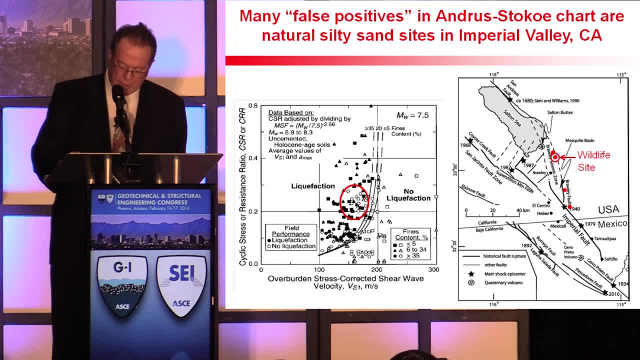 That liquefied extensively In the 1989 Loma Prieta earthquake. However, In 1910. This wildlife site Was subjected to an earthquake Compatible to Loma Prieta, Which generated only a small Poor pressure In the liquefiable layer. 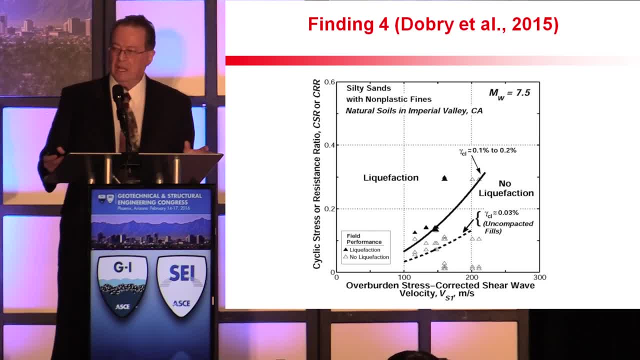 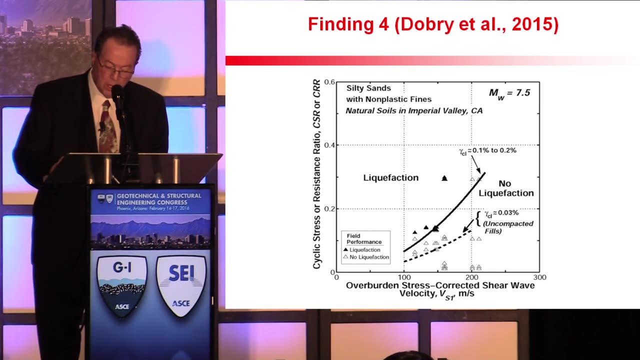 So Again, We took all case histories In the Andrews and Stokke database Located in the imperial valley, Which were either clean Or not, And plotted them on the same CSR versus VS1 plot. We were able to fit this parabola. 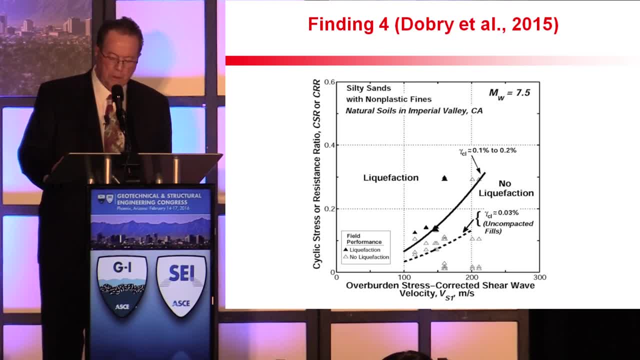 The solid line Separating liquefaction From no liquefaction, Which corresponds to a cyclic strain Much greater than the 0.03% We had found before For the uncompacted fields. That is The cyclic shear strain needed for triggering. 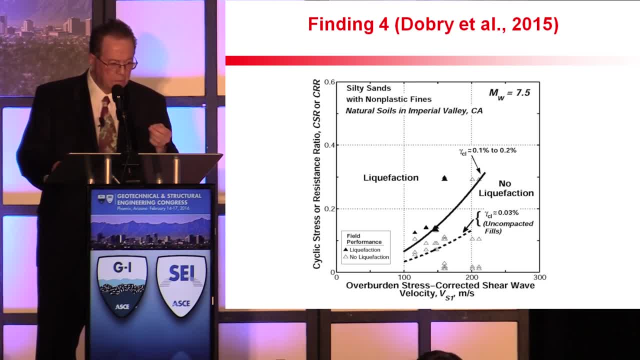 In the imperial valley sands Is of the order of 0.1 to 0.2%- Four times greater, With the corresponding Solid line parabola Playing so much higher Than the parabola for the uncompacted fields. 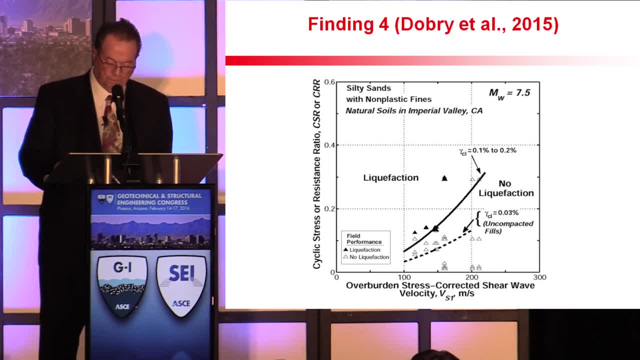 Which is shown on the screen By the dash line below. In fact, The CRR- The liquefaction resistance needed for triggering In the imperial valley, Is almost exactly twice That of a recent uncompacted field Of equal VS1.. 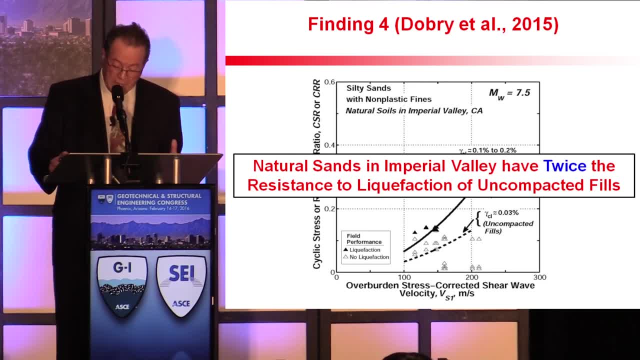 With the corresponding number Four. This would explain the false positives Of the chart By heavy pre-shaking Due to previous earthquakes. It also suggests That a given family of sites And sand layers Subjected to a similar geologic 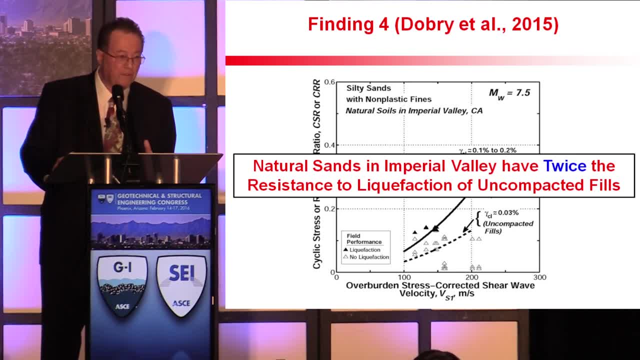 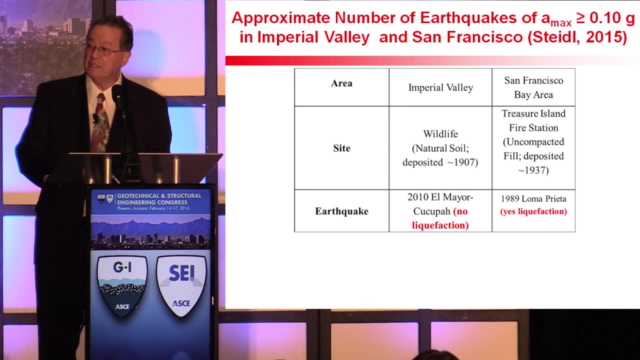 And seismic environment, Like in this case, May be characterized by a regional Liquefaction chart. In this particular environment, To understand better what happened, We focus on the liquefiable Layer at the wildlife site, Which seems to have been. 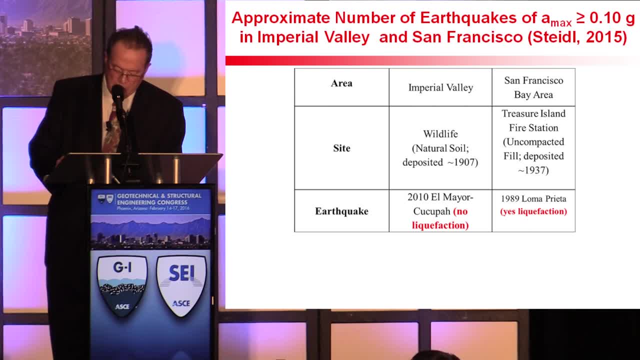 Deposited by flooding In 1907. So the layer must have had a fabric Similar to the hydraulic field Immediately after deposition. Then We took a comparable silty sand site In the San Francisco bay area, The Treasure Island. 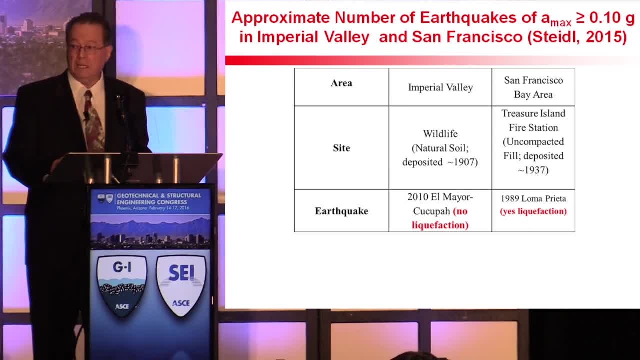 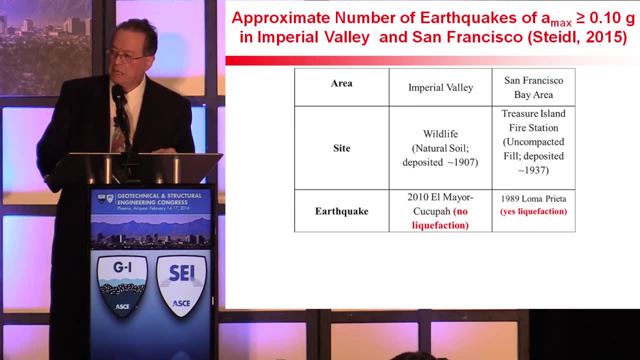 Which was a fire station site That did liquefy in 1989. And which had been Deposited artificially As a hydraulic field In the 1930s, That is, half a century Before the earthquake, Dr Steidle. 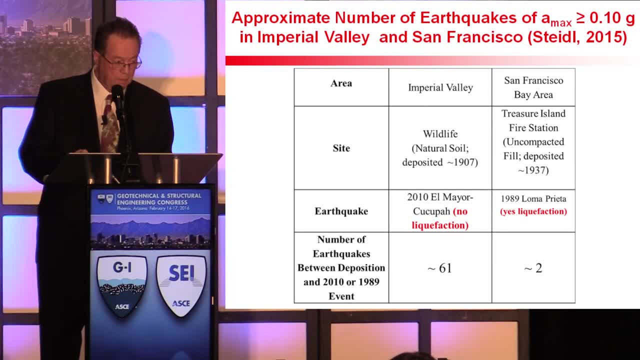 A seismology at UC Santa Barbara Helped us understand What happened. He went to the earthquake catalog And counted a total Of about 61 earthquakes Between a peak ground acceleration Greater than .10 G At wildlife. Between deposition: 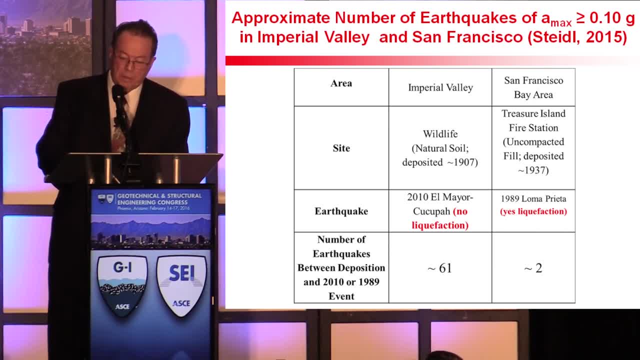 And the 2010 earthquake, When the site had a shaking Similar to Loma Prieta, But did not experience liquefaction. Dr Steidle then repeated The same earthquake, counting For the Treasure Island site, And found that there had been 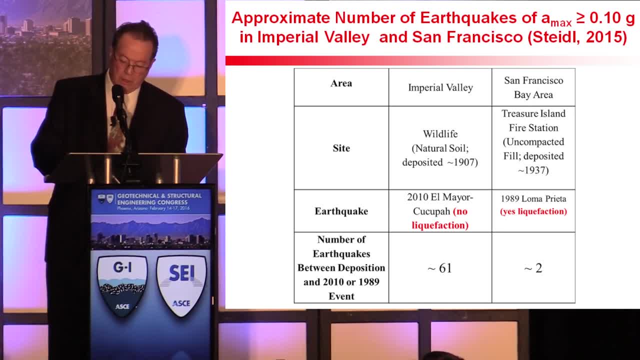 Only two earthquakes Of more than .10 G, Which seems to explain Why at Treasure Island, The layer still behaved As a recent sand fill in 1989. While at wildlife, The layer behaved as a heavily Pre-shaking sand of increased resistance. 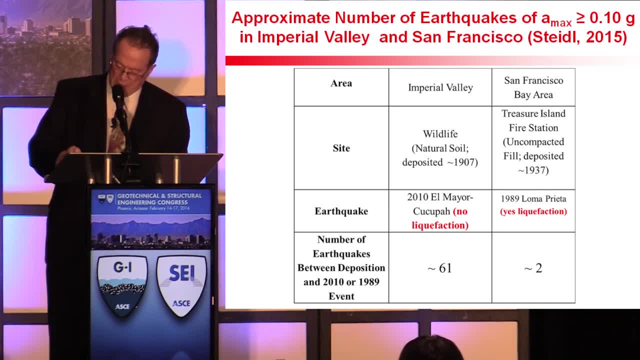 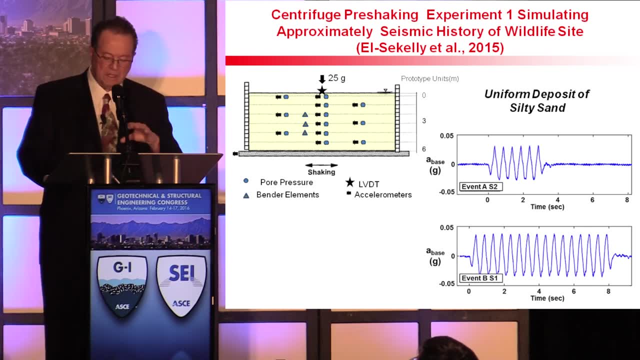 In 2010.. We decided to investigate further The influence of pre-shaking On liquefaction resistance Through a series of centrifuge And large scale experiments. We did Three centrifuge tests And one large scale test Using two sands. 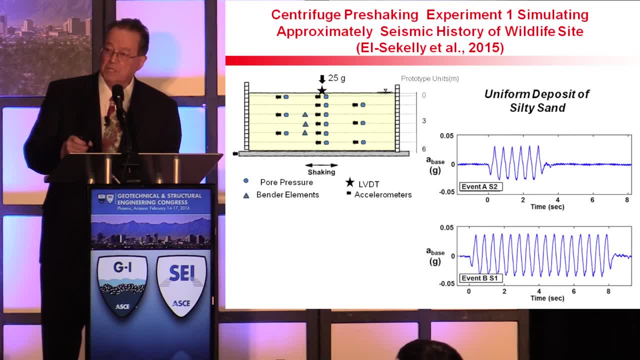 A clean sand and a silty sand. In all four experiments, We placed a deposit of about six meter thickness And subjected it to several dozen shakings, Using different patterns And simulating In an idealized way The seismic history of a sand. 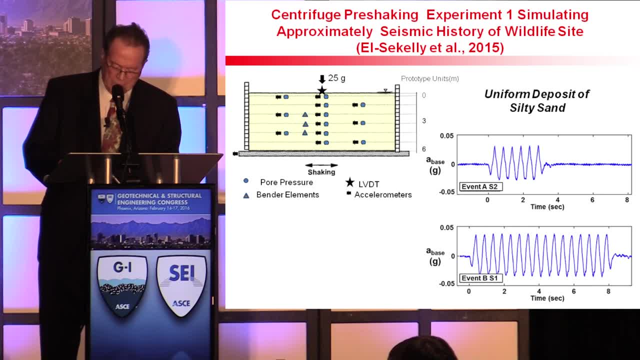 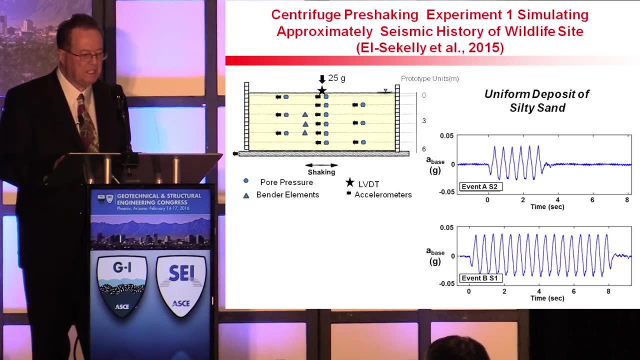 Located, for example, in the Imperial Valley Or in another very seismic area Experiment, one That you see on the screen And that approached most closely, But still in a very crude way, The situation at wildlife. Specifically, We applied a total of 66 shakings. 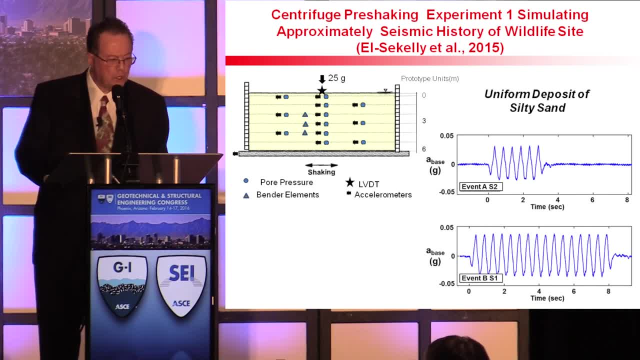 Of which most corresponded To this short duration. A, The one with five cycles at the top And a few shakings, Correspond to this much longer duration: 15 cycle duration. Event B: Events B: Were expected to liquefy the deposit. 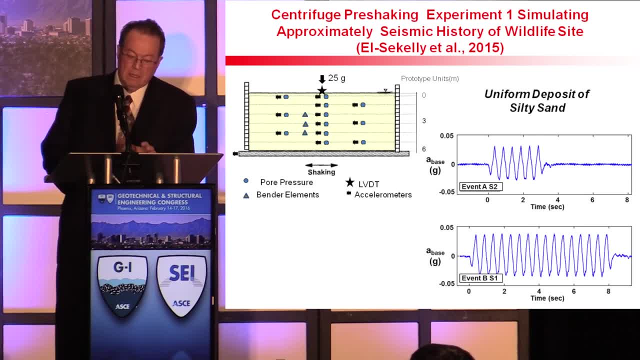 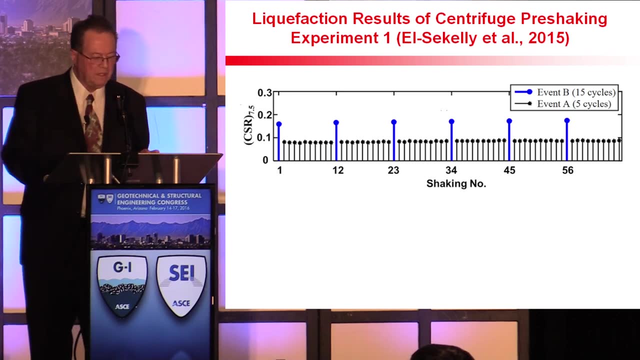 At least at the beginning of the test, While events- A Many of them- Represented many local pre-shaking events That have been observed at the site, Which typically generate poor pressures But not liquefaction. Here you see The sequence of the 66 shakings. 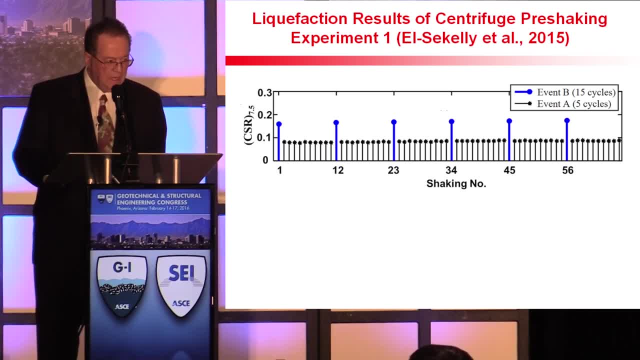 In this experiment one. The ordinate of the plot Is CSR 7.5. Normalized to 7.5. Magnitude earthquake. In order to account For the different durations Of events A and B, Events B Are the blue vertical lines. 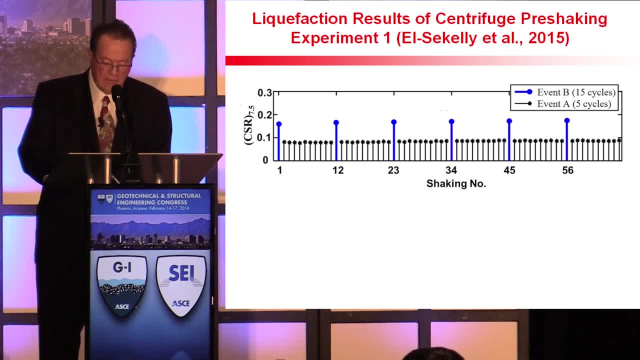 Six events in total, And the events A Are the 60. Black vertical lines. This bottom plot Shows, for the Each of the 66 events, The maximum poor pressure ratio Measure anywhere In the deposit At the end of shaking RU max. 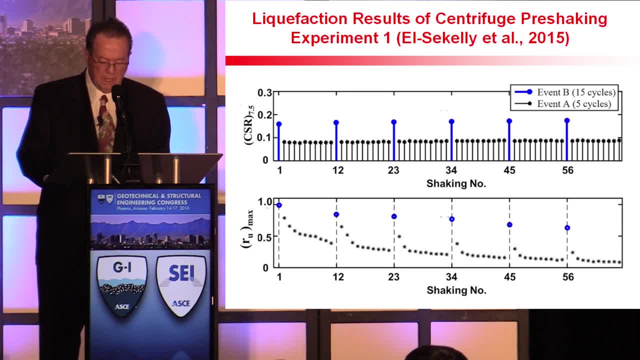 This is a fascinating plot. The first event B Labeled shaking 1.. Number 1. Induced an RU max of 1.0. Liquefying the deposit. The first Blue dot At shaking number 1.. 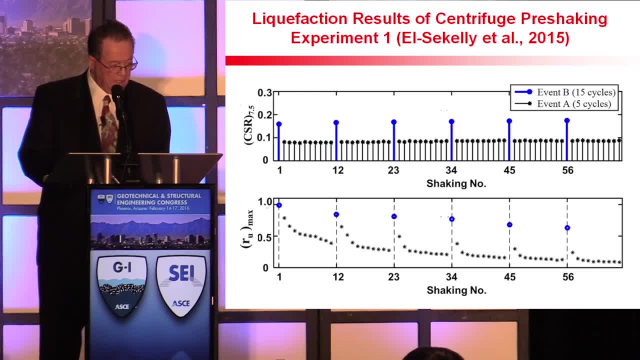 50 events later, Or 56 events later, Shaking number 56.. Which is also a blue dot, Is also an event B- Did not induce liquefaction, With RU max Being 0.6.. This event B, Shaking 56.. 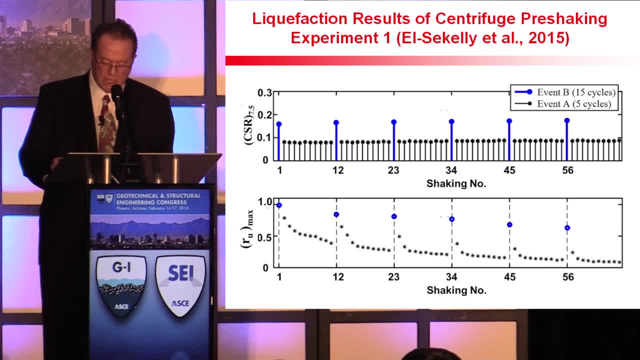 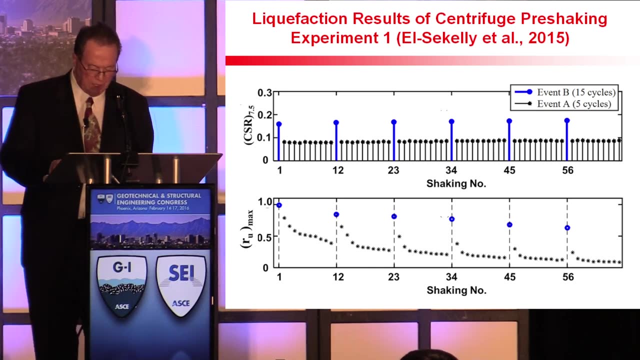 Is of special interest As it approaches the situation At wildlife At the time of the 2010 earthquake, Which also did not cause liquefaction. The poor pressure responses For event A Are also illuminating: The poor pressure ratio. 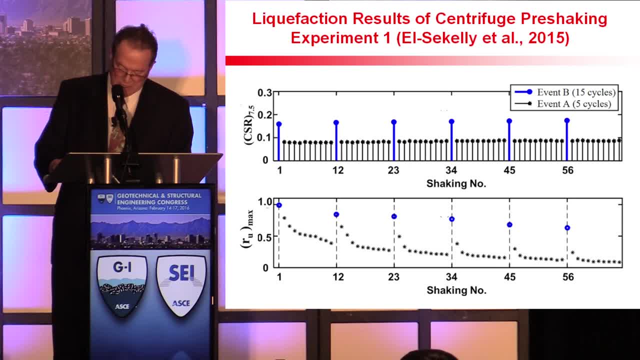 Decreases fast Within any sequence of 10 events A- I cannot show you this- But jumps to a much higher value Immediately after an event B, And then it starts Decreasing again, Canceling the effect of the event B. 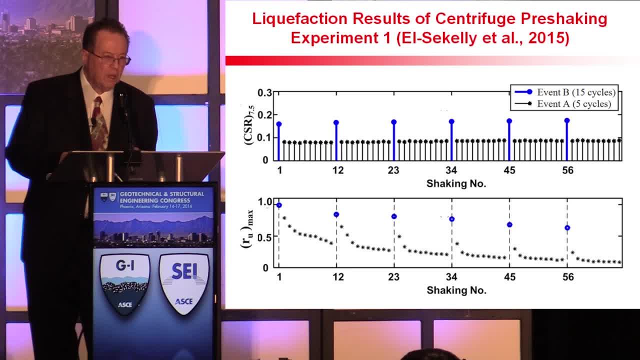 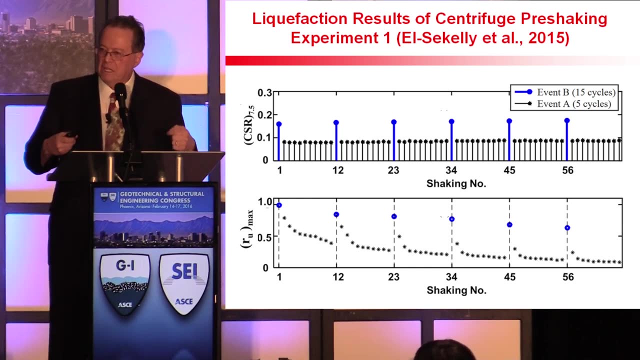 After 2 or 3 events A. Therefore, This is, In terms of liquefaction resistance, Is a Two steps forward, One step backward Process, With a net result In the long run Of a significant increase In liquefaction resistance. 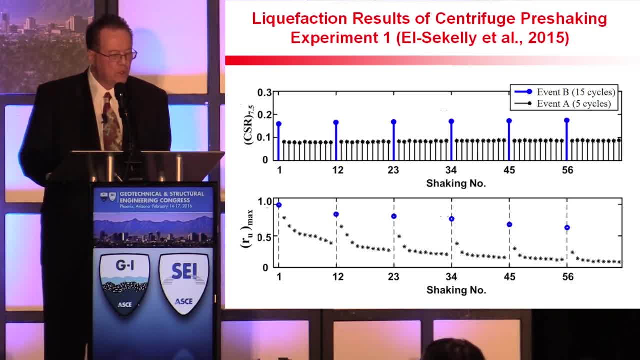 You can see that the events A Have much higher Poor pressure ratios Between events 2 and 12.. 2 and 11. That between events 46 and 55. I mean The net result. We measure The shear wave velocity of the soil. 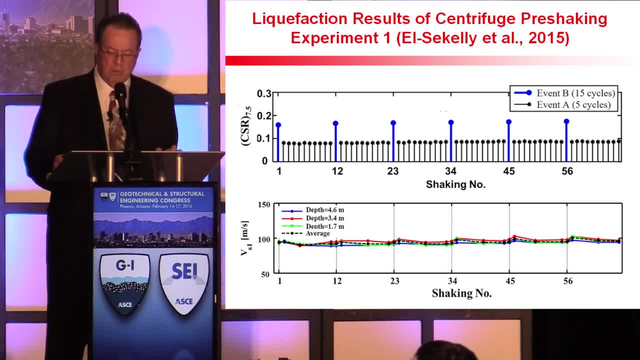 Between events with bended elements, And the pattern is extremely simple And baffling. While the liquefaction resistance Was varying dramatically, Going up and down, But with the sun being clearly stronger After 50 or 60 shaking, The shear wave velocity almost did not change. 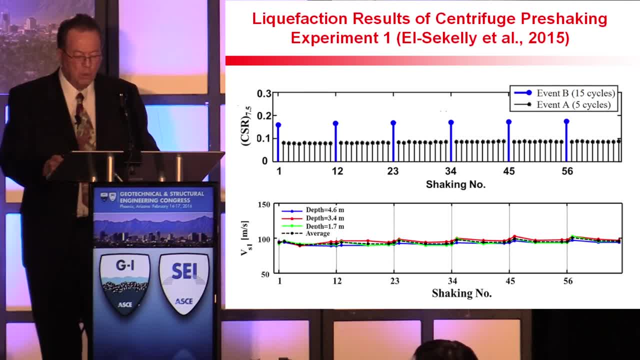 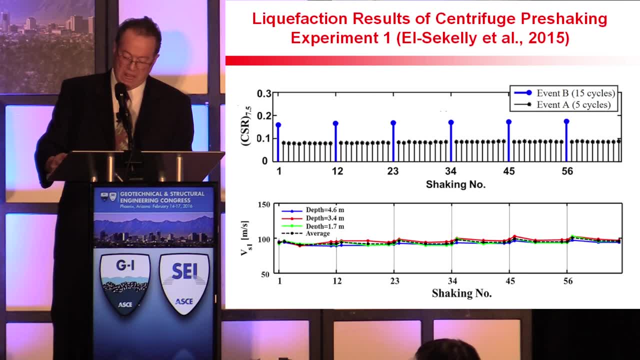 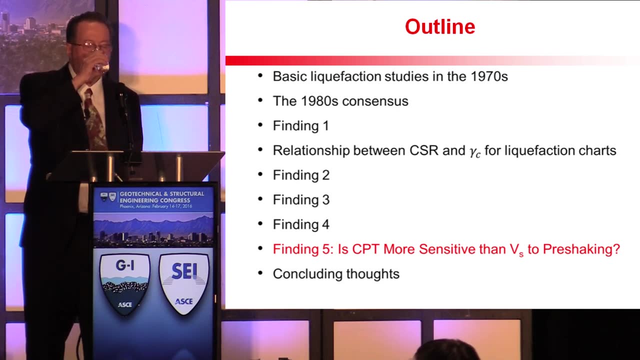 The value of the S1. Of the silty sun Was about 100 meters per second At the beginning, Until 100 meters per second At the end. And this Brings me to our finding Number 5.. Which is the answer? 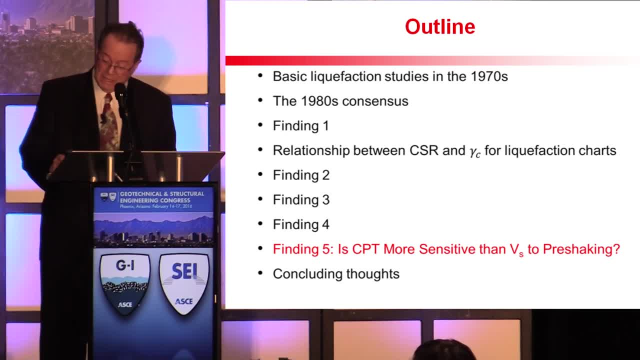 To the following question: Is the CPT More sensitive to pre-shaking Than VS, Thus reflecting better the increase we see In liquefaction resistance Over the long run? This should be the case Because the CPT is more sensitive. 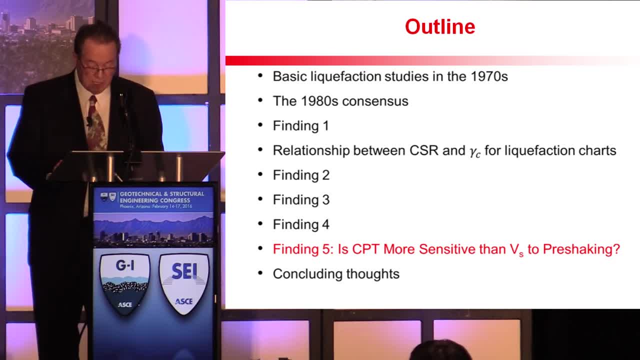 To increases in relative density And is also more sensitive To the lateral stresses That presumably also increase During the pre-shaking. But we wanted to check this conclusion In our own research. We did that by taking CPT measurements In the full scale test we conducted. 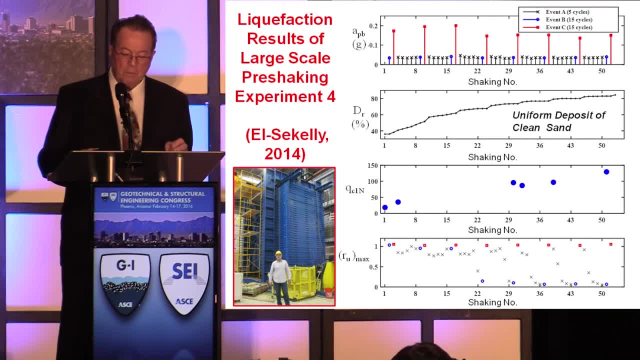 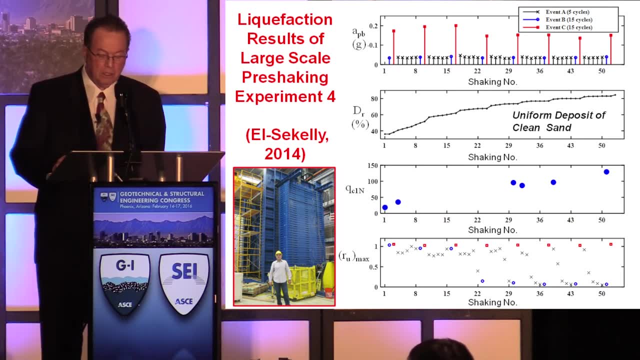 As part of our 4 experiments. This experiment: 4. Done on clean sand At the University of Buffalo, In the 6 meter tall laminar box Which is shown in the photo, Where you can also see Dr Elzekely. 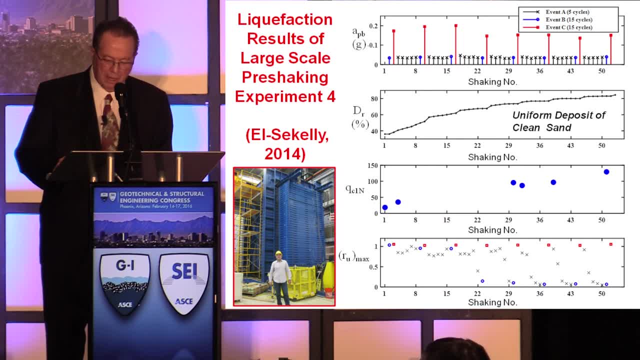 Who is a tall fellow, Despite the appearances. The 52 shakings are shown In the plot at the top, Where We have plotted The peak base acceleration For each shaking: A sub pb. One difference with the test. 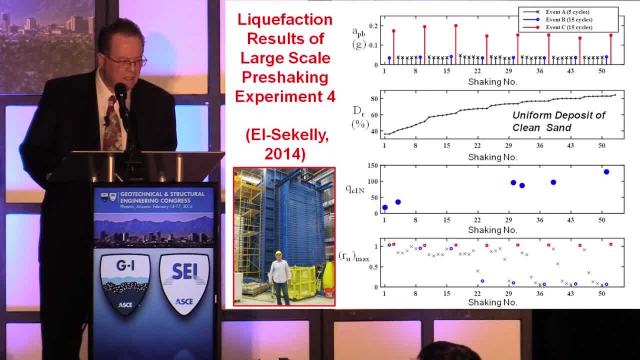 I showed you before Is that now we have some very strong events C: 1,2,3,4,5,6,7.. 8 events C, Which are the red lines, The red vertical lines. These are 15 cycles of 0.2 g. 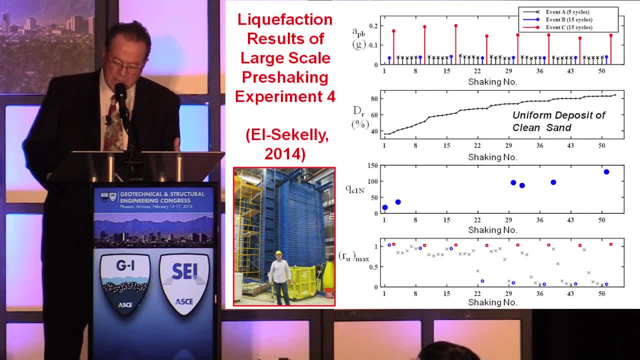 This is gigantic. And this event C Always liquefies the soil. If you go to the bottom plot, You see the red open squares And they are all at 1.0.. They always liquefy the soil. The pattern of pore pressure in the bottom plot. 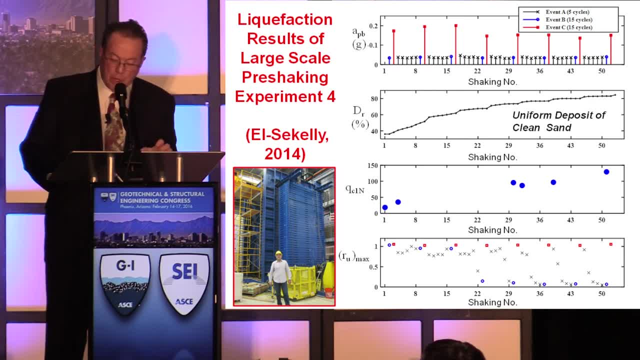 For Ru max Is complicated, But in fact it also follows The same general rule of two steps forward, One step backward. As you can see With the blue dots And the black dots, at the end They are much smaller than at the beginning. 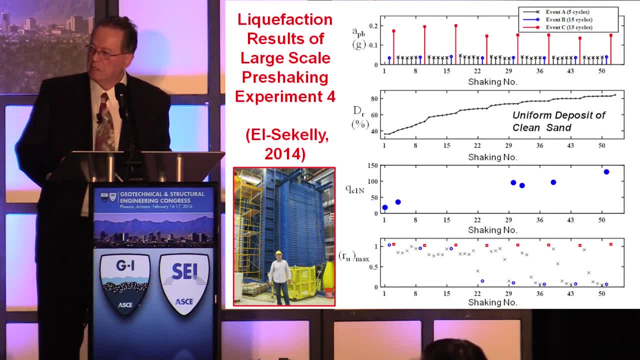 Okay, When everything is said and done, There was an increased liquefaction resistance. Now The deposit was significantly densified By all these shakings. If you go to the second plot, You can see the relative density At the beginning. 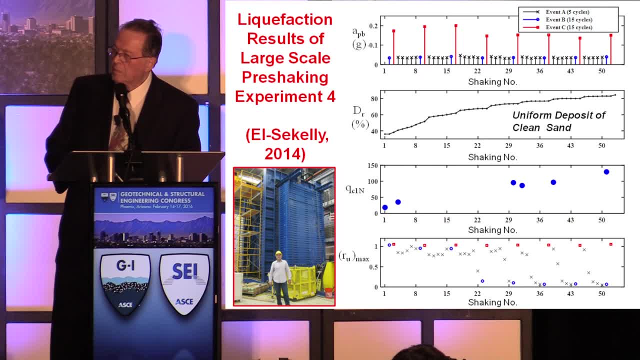 Was less than 40% And it was more than 80% at the end. And the third plot From the top Which shows the point resistance Normalized, point resistance Qc1n. It had a huge increase, It was about 17.. 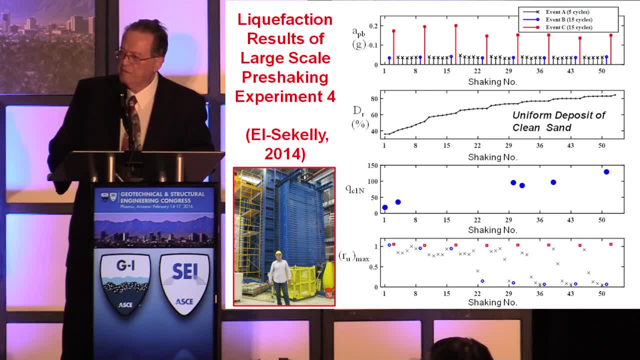 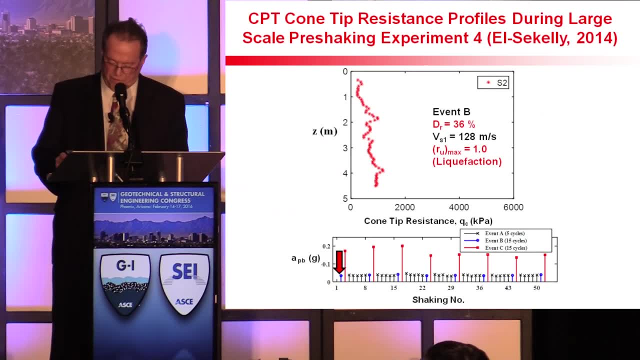 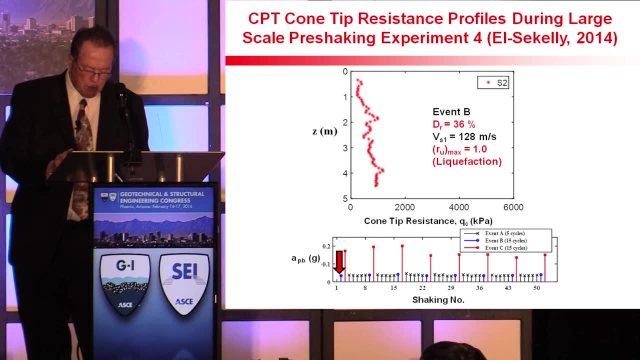 At the beginning And it was 130 at the end. This is a factor of 8.. Let me walk you through Three CPT profiles, Measured before Three events B. Immediately before three events B Using the pore: pressure responses. 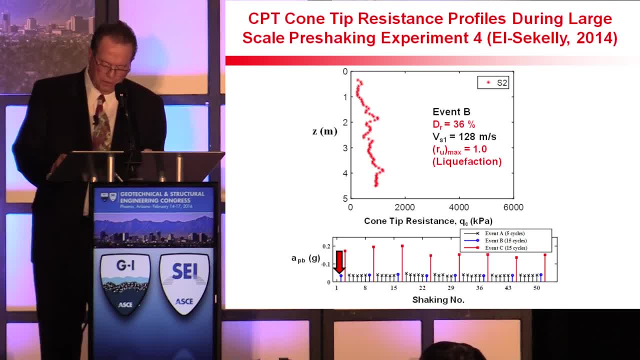 To those events. B In order to show you How the liquefaction resistance was shaking And how the corresponding CPT point resistance And also the Vs And the relative density were changing all at the same time. This is the first Baseline CPT measurement. 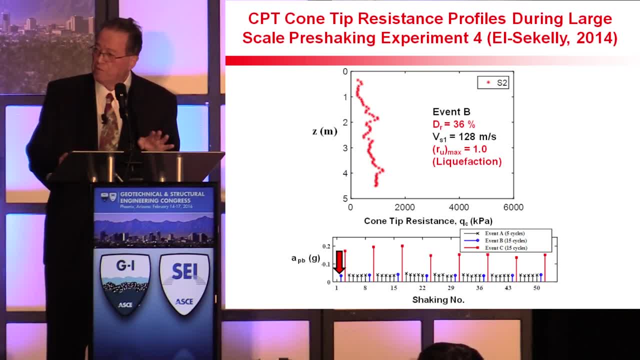 Done before any shaking And immediately before the first Event, which was An event B. The relative density was 36%, Vs1 was 128 meters Per second. The event B immediately afterwards Did liquefy the deposit: Ru max equal 1.0.. 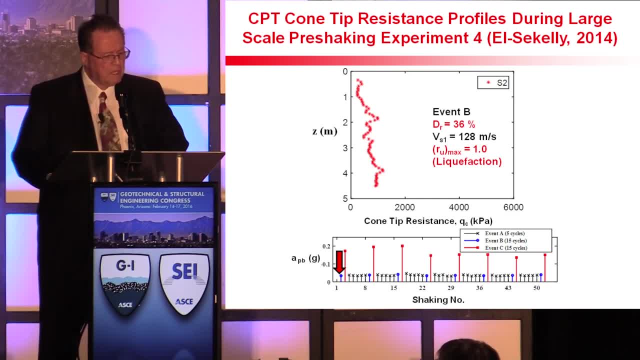 And to fix ideas. If you go to a depth of 2.5 meters, Which is about mid depth, The point resistance of the cone Is about 500 kPa. Keep that in mind And the point resistance of the cone. 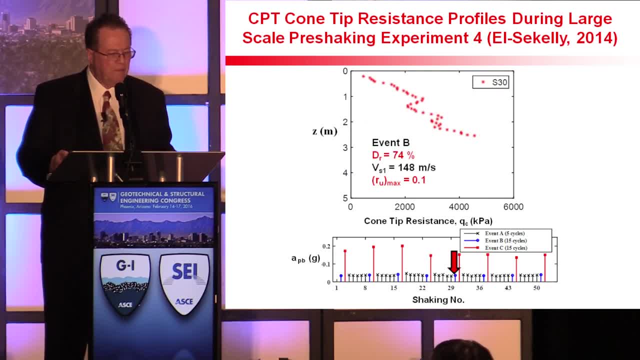 Is about 500 kPa, 30 events later, Shaking number 30. The relative density Has increased a lot, From 36 to 74%. The shear wave velocity Has increased a little bit, About 10-15%. 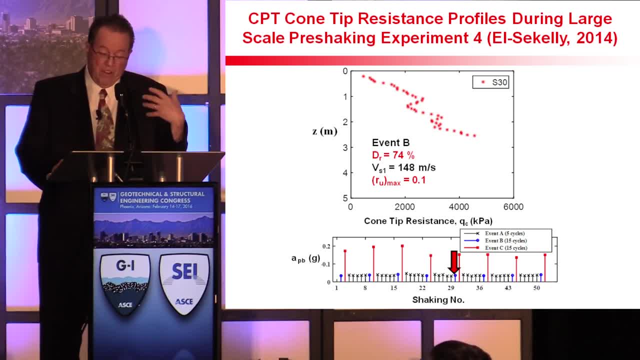 From 128 to 148 meters per second. The deposit is now building up A very small pore pressure ratio Of 0.1. for the subsequent event B Collapse from 1.0 to 0.2. Which means it has a much higher. Liquefaction resistance And The CPT at 2.5 meters Has also had A huge increase. In CPT At 2.5 meters it was 500 kPa, Now it's 3000. That's a factor of 6.. 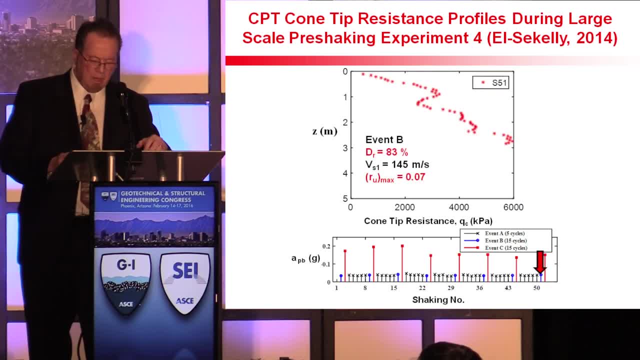 And finally Let's jump to shaking number 51.. At the end of the experiment, Relative density has to continue to increase a bit, From 74 to 83.. Shear wave velocity is not changing anymore. Deposit again built up A very small pore pressure ratio. 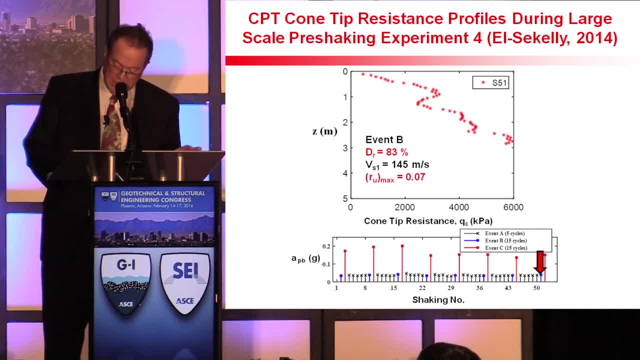 In this case 0.07, 0.1.. Instead of 1.0 at the beginning, And the CPT at 2.5 meters Has continued to increase: 500, 3000.. Is now 4000.. KPa, A factor of 8. Compared with the initial point, resistance Of the CPT. Now I'm saying that this factor of 8. Between 500 kPa And 4000 kPa At the end of the experiment. 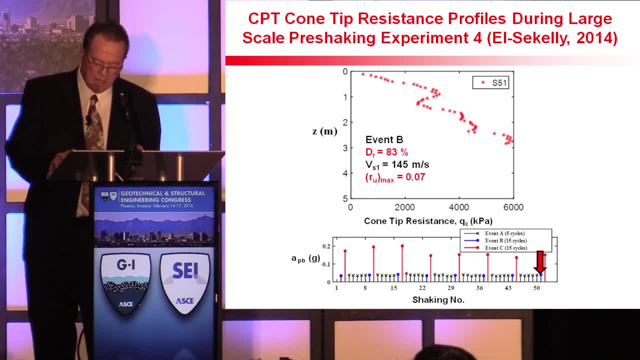 Necessarily represents the field conditions, As the measure CPT May have been influenced by the wall Of the lamina box, But clearly there was a tendency For the CPT to increase very rapidly And if the factor in the field 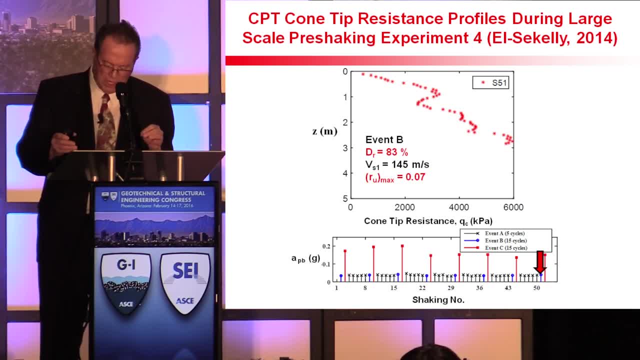 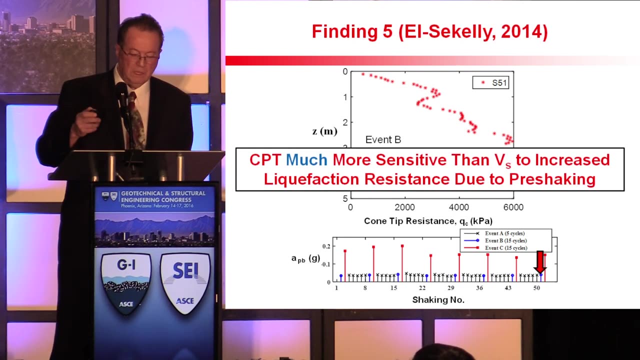 Is only 4 or 5. Instead of 8.. This still represents a huge increase in the CPT Caused by soil densification And higher lateral stresses Produced by the pre-shaking process. Therefore, This is our finding number 5.. 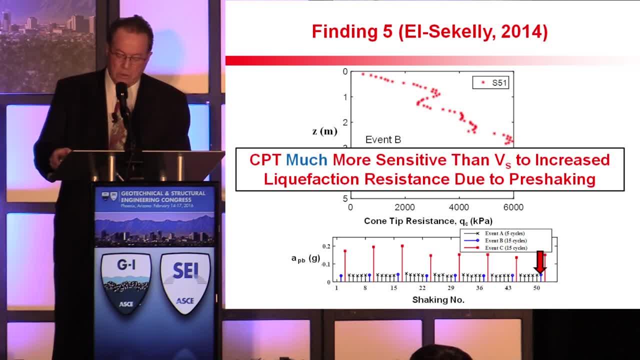 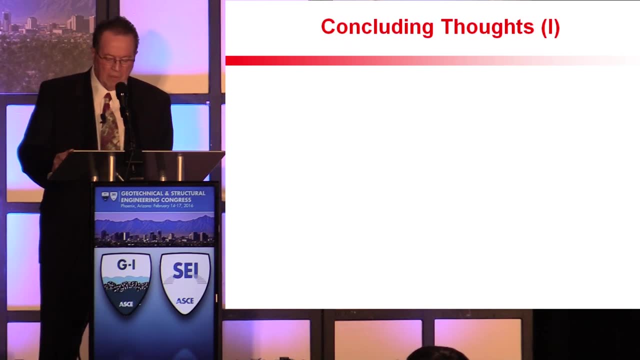 Which is really a confirmation Of what other people had already found And that we expected. The CPT point penetration resistance Is much more sensitive Than shear wave velocity To the increased liquefaction resistance Due to pre-shaking. Let me add some concluding thoughts. 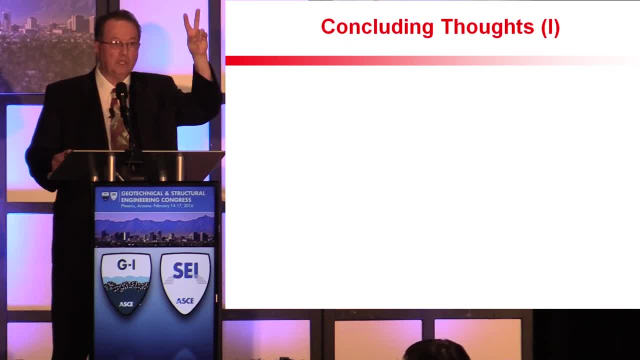 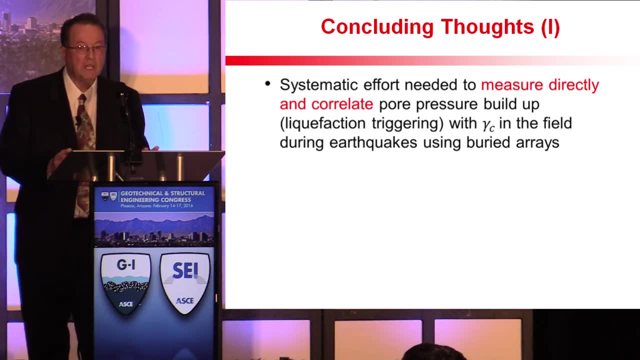 From this research I'm down to my last two slides. I would like to make two general points In this first slide. My first point Is a recommendation That we should start a systematic effort To measure directly The cyclic shear strain. 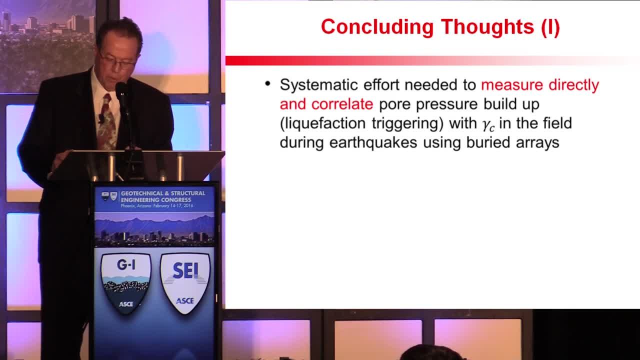 In the field during earthquakes, As the sand layers build up For pressures and trigger liquefaction. By using existing Or still to be built With varied arrays of accelerometers And piezometers, The technology exists. Several groups have already shown. 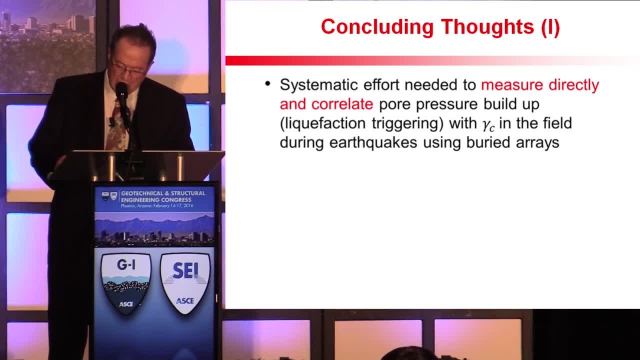 How this can be done Using system identification, And this would allow Building up a database Where pore pressure build up Is directly correlated to shear strain For future applications. We already know that pore pressures Are more uniquely correlated to gamma sub C. 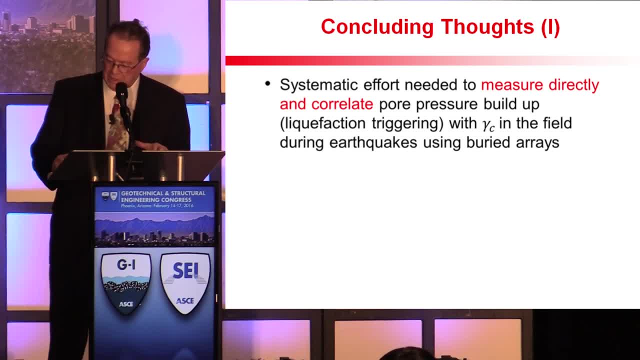 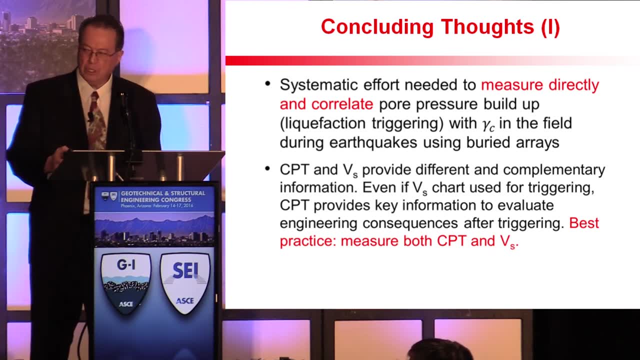 Than to cyclic stress ratio. Therefore, let's put this knowledge To use. My second point Relates to the use in the field Of the cone penetration And shear wave velocity methods, Which provide different pieces of information That complement each other. 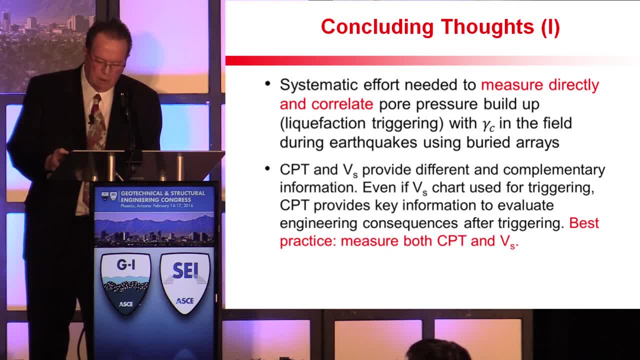 Even if a decision is made To use a VS chart for triggering evaluation, Clearly the CPT provides Additional key information To evaluate engineering consequences After triggering. at the very least, The best practice Is just to measure both CPT And CPT performance. 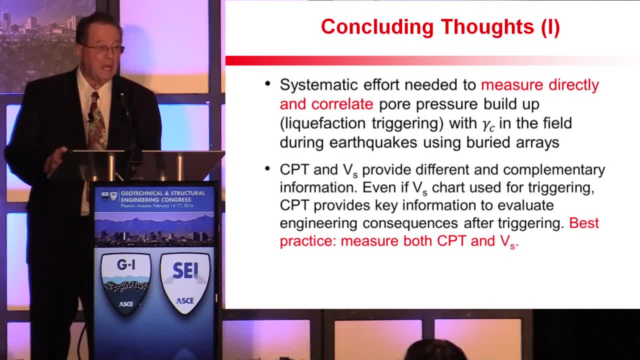 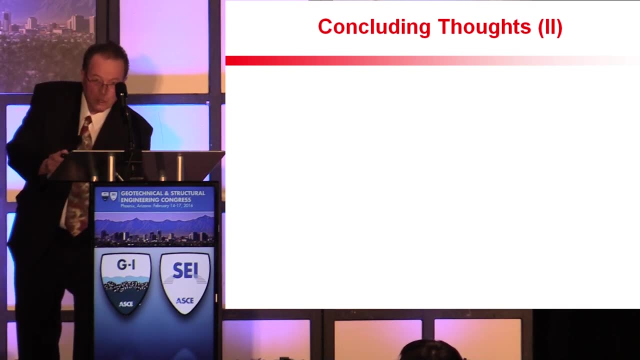 We are not alone in suggesting this. A similar recommendation Has also been made, between others, By Dr Schneider and Moss And by last year's seed lecturer, Dr Peter Robertson, In this second And last slide Of my presentation.